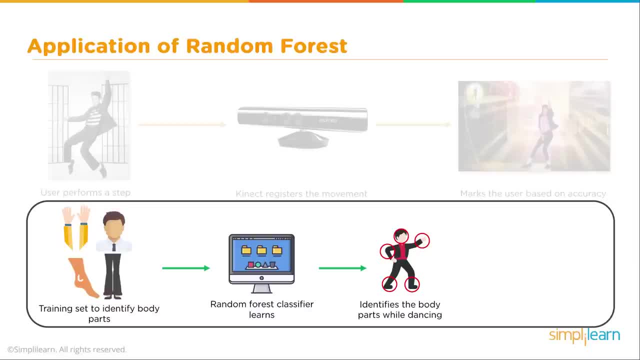 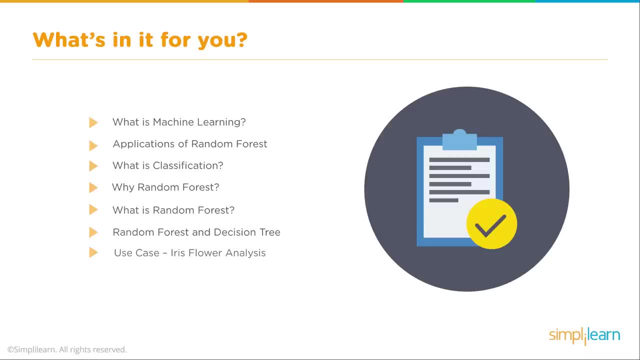 It's able to represent that in a computer format And then, based on that, it scores the game. and how accurate you are as being Elvis Presley or Prince, and you're dancing. Let's take an overview of what we're going to cover today. What's in it for you? 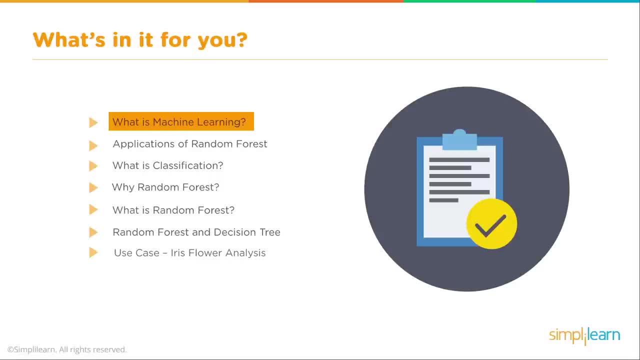 We're going to start with what is machine learning? We're not going to go into detail on that. We're going to specifically look at how the Random Forest fits in the machine learning hierarchy. Then we're going to look at some applications of Random Forest. 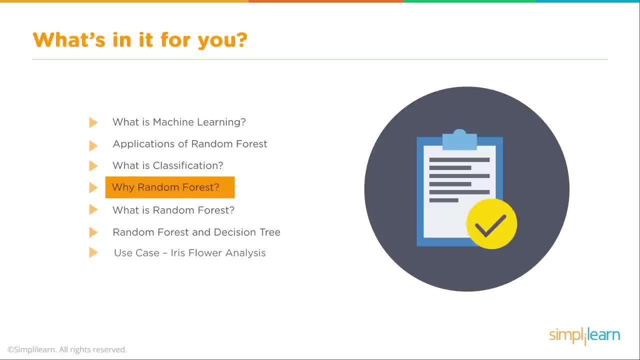 What is classification, which is its primary use? Why use Random Forest? What's the benefits of it And how does it actually come together? What is Random Forest? And then we'll get into Random Forest and the decision tree. That's like the final step in how it works. 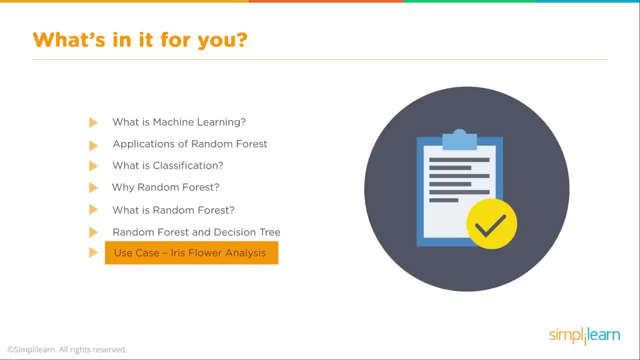 And finally, we'll get some Python code in there and we'll use the case, the Iris Flower Analysis. Now, if you don't know what any of these terms mean or where we're going with this, don't worry, We're going to cover all the basics. We're going to cover the basics. 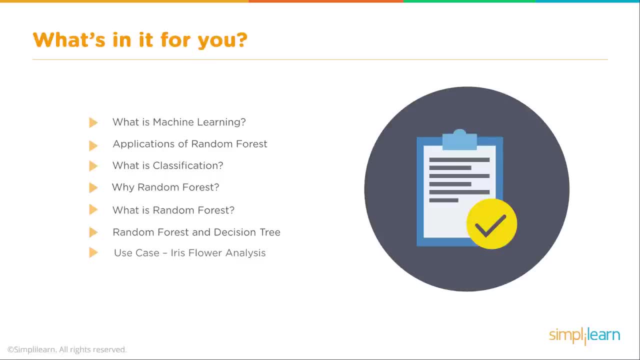 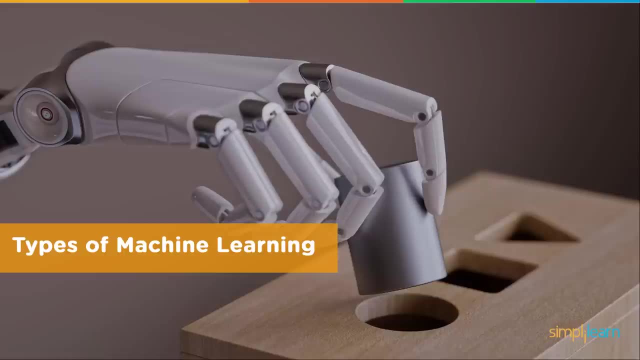 And have you up and running and even having doing some basic script in Python by the end. Let's take a closer look at types of machine learning. Specifically, we're going to look at where the decision tree fits in with the different machine learning packages out there. 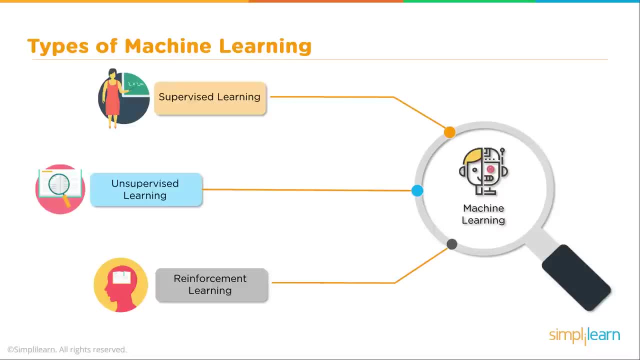 We'll start with the basic types of machine learning. There's supervised learning, where you have lots of data and you're able to train your models. There's unsupervised learning, where it has to look at the data and then divide it based on its own algorithms, without having any training. 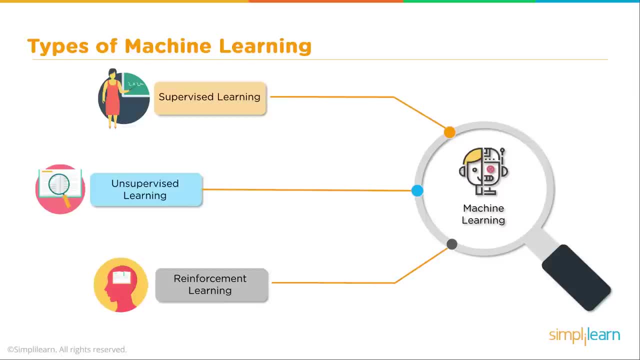 And then there's reinforcement learning, where you get a plus or negative if you have the answer correct. This particular tool belongs to the supervised learning. Let's take a closer look at that: what that means in supervised learning. Supervised learning falls into two groups: classification and regression. 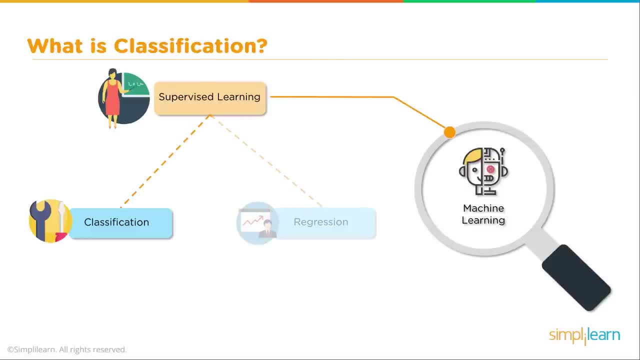 We'll talk about regression a little later and how that differs. This particular format goes underneath classification, So we're looking at supervised learning and classification in the machine learning tools. Classification is a kind of problem where the outputs are categorical in nature, like yes or no, true or false or zero or one. 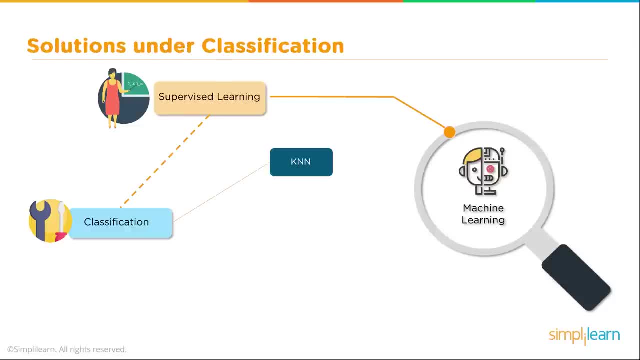 In that particular framework there's the KNN, where the NN stands for nearest neighbor knave Bayes, the decision tree, which is part of the random forest that we're studying today. So why random forest? It's always important to understand. 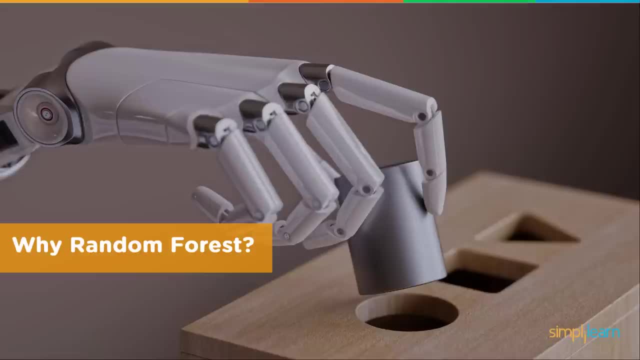 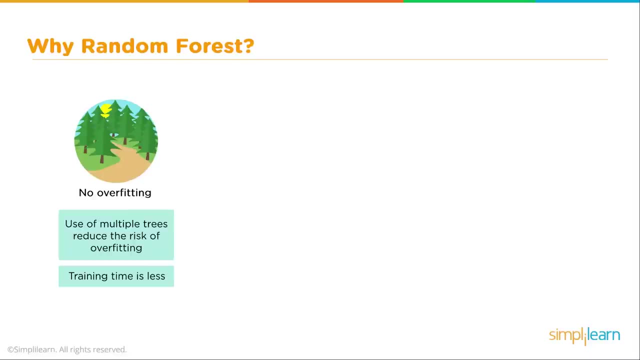 why we use this tool over the other ones. What are the benefits here And so with the random forest? the first one is: there's no overfitting Use of multiple trees. reduce the risk of overfitting. Training time is less. 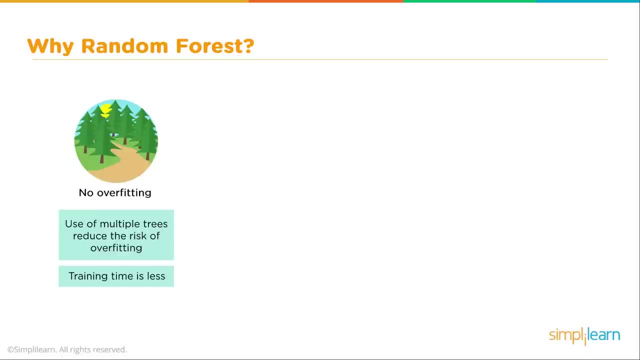 Overfitting means that we have fit the data so close to what we have as our sample that we pick up on all the weird parts And, instead of predicting the overall data, you're predicting the weird stuff which you don't want. High accuracy Runs efficiently on large database. 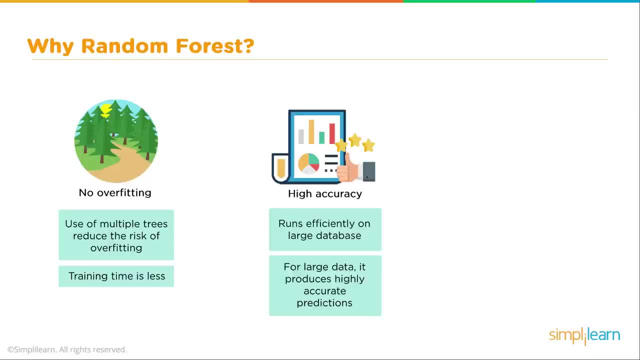 For large data. it produces highly accurate predictions. In today's world of big data, this is really important And this is probably where it really shines. This is where why random forest really comes in. It estimates missing data. Data in today's world is very messy. So when you have a random forest, 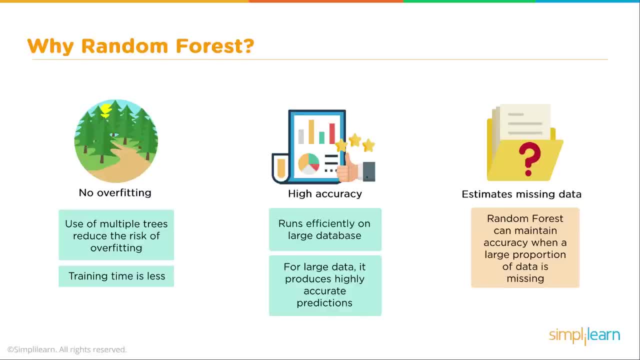 it can maintain the accuracy when a large proportion of the data is missing. What that means is if you have data that comes in from five or six different areas and maybe they took one set of statistics in one area and they took a slightly different set of. 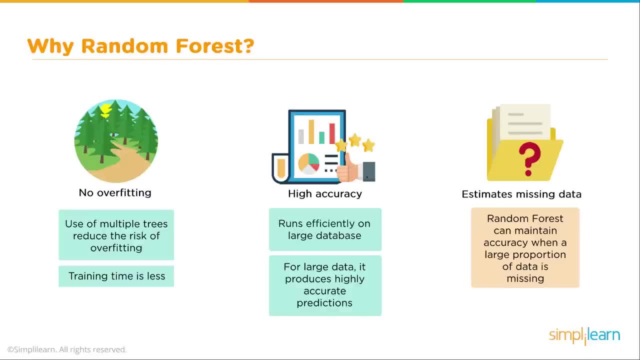 statistics in the other. so they have some of the same shared data, but one is missing, like the number of children in the house, If you're doing something over demographics, And the other one is missing, the size of the house. It will look at both of those separately and build two different trees. 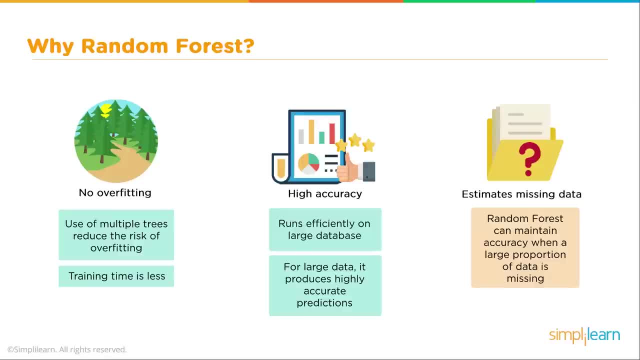 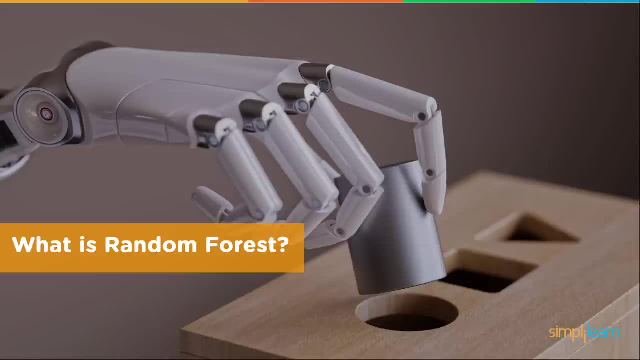 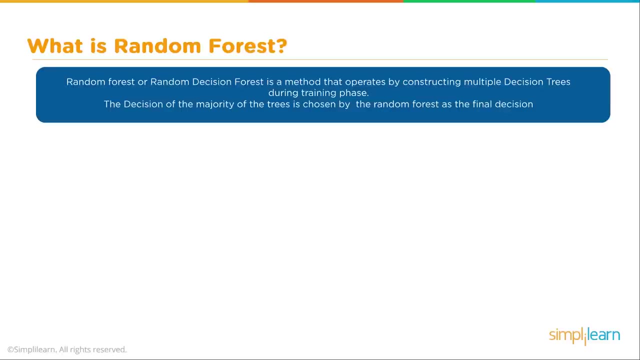 And then it can do a very good job of guessing which one fits better, even though it's missing that data. Let us dig deep into the theory of exactly how it works And let's look at what is random forest. Random forest or random decision forest is a method that operates by constructing multiple 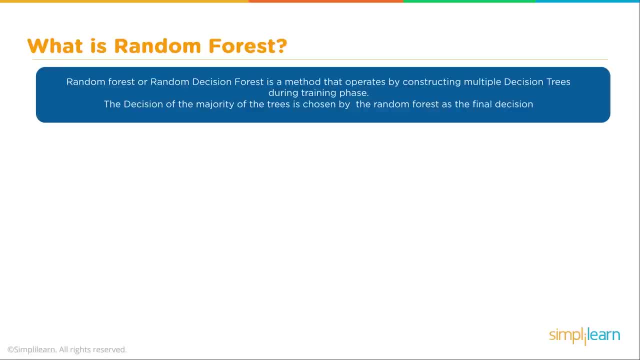 decision trees. The decision of the majority of the trees is chosen by the random forest as the final decision. And this we have some nice graphics here. We have a decision tree and they actually use a real tree to denote the decision tree. 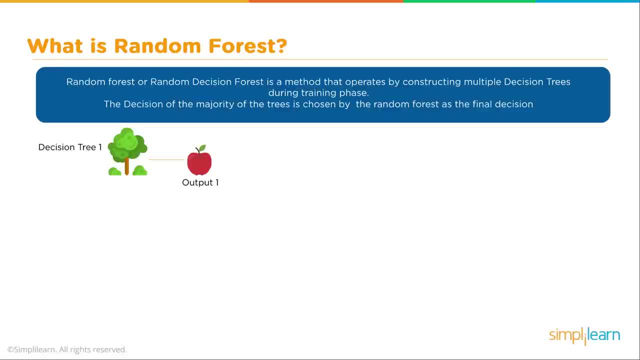 which I love, And given a random, some kind of picture of a fruit, this decision tree decides that the output is it's an apple. And we have a decision tree two, where we have that picture of the fruit goes in and this one decides that it's a lemon. 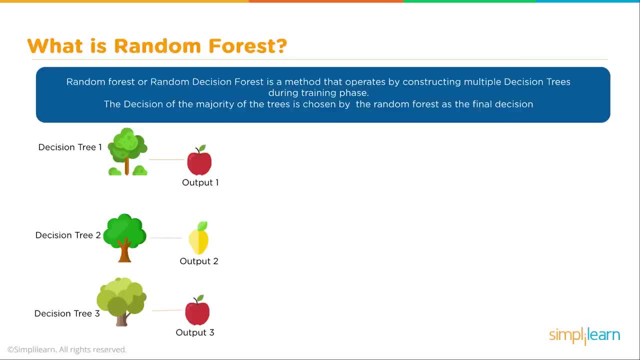 And the decision tree three gets another image and it decides it's an apple. And then this all comes together And what they call the random forest. And this random forest then looks at it and says: OK, I got two votes for apple, one vote for lemon. 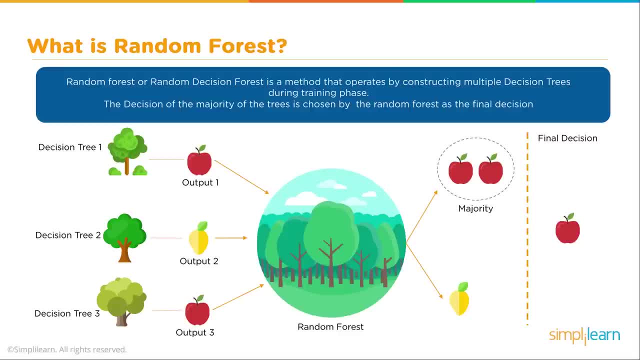 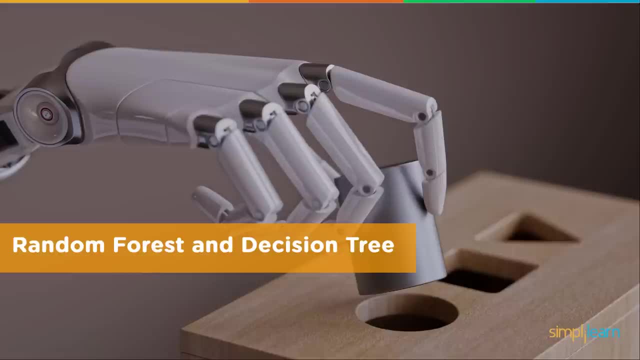 The majority is apples, So the final decision is apples. To understand how the random forest works, we first need to dig a little deeper and take a look at the random forest and the actual decision tree and how it builds that decision tree. In looking closer at how the individual decision trees work, 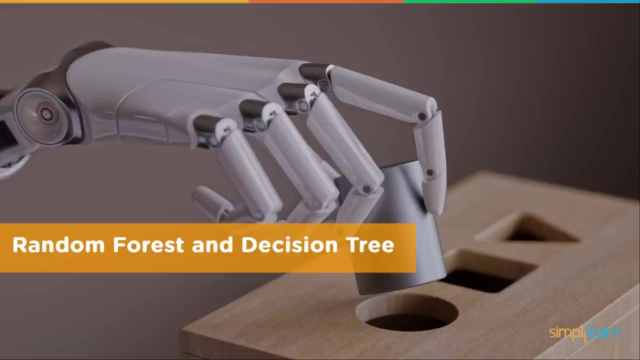 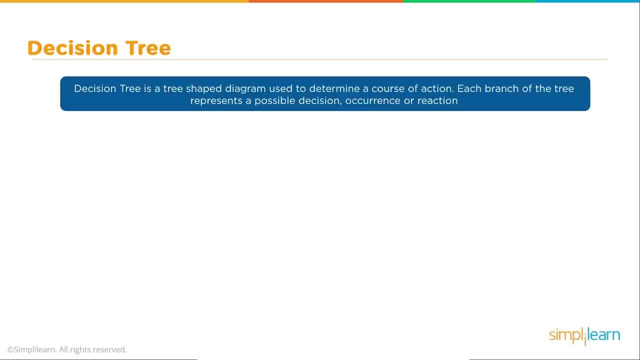 we'll go ahead and continue to use the fruit example, since we're talking about trees And for us, a decision tree is a tree shaped diagram used to determine a course of action. Each branch of the tree represents a possible decision occurrence or reaction. 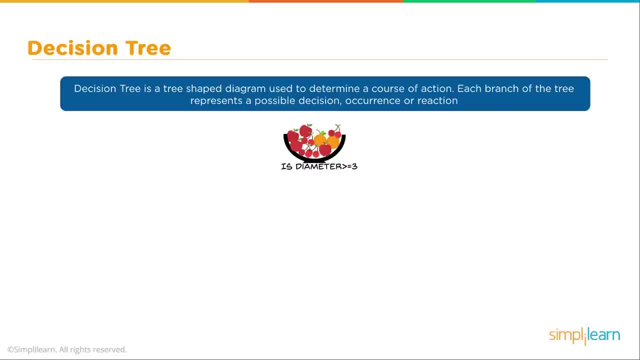 So in here we have a bowl of fruit And if you look at that it looks like they switch from lemons to oranges. We have oranges, cherries and apples, And the first decision of the decision tree might be is the diameter greater than or equal to three. 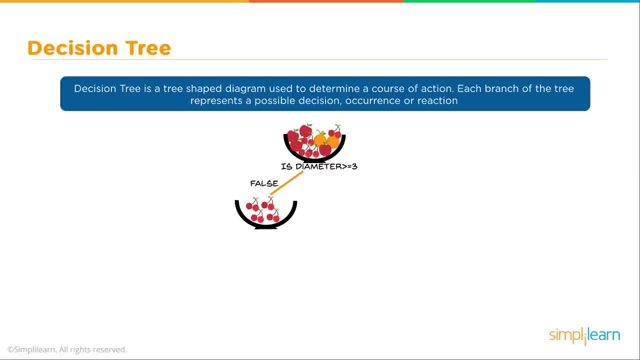 And if it says false, it knows that they're cherries because everything else is bigger than that. So all the cherries fall into that decision. So we have all that, All that data we're training. we can look at that. We know that that's what's going to come up. 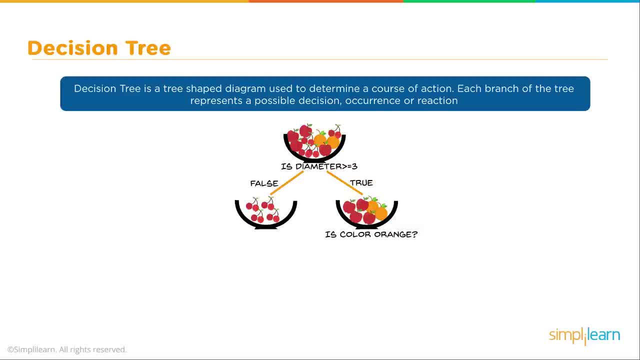 Is the color orange. Well it goes. hmm, orange or red? Well, if it's true, then it comes out as the orange, And if it's false, that leaves apples. So in this example, it sorts out the fruit in the bowl. 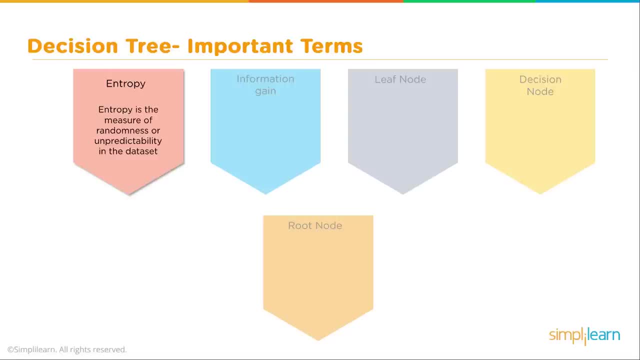 or the images of the fruit, A decision tree. these are very important terms to know because these are very central to understanding the decision tree and when working with them. The first is entropy. Everything on the decision tree and how it makes those decisions is based on entropy. 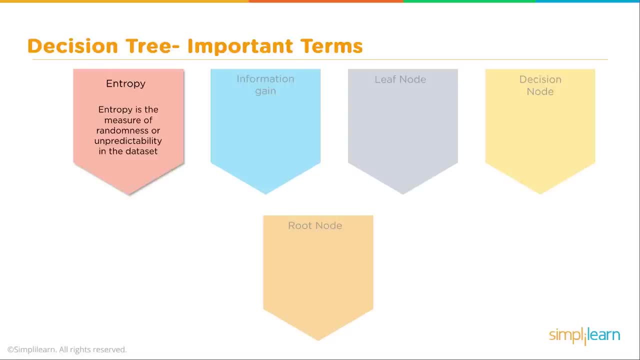 Entropy is a measure of randomness or unpredictability in the data set. Then they also have information gain, the leaf node, the decision node and the root node. We'll cover these other four terms as we go down the tree, But let's start with entropy. 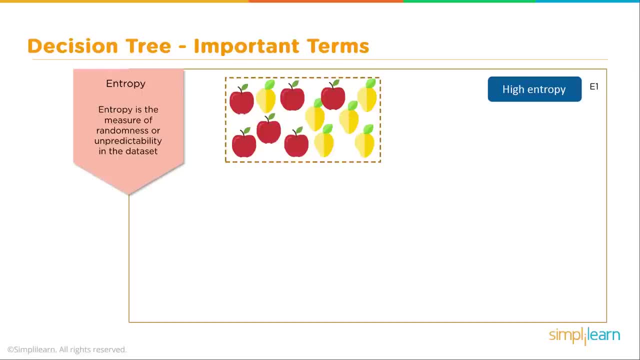 So, starting with entropy, we have here a high amount of randomness. What that means is that, whatever is coming out of this decision, that data set is going to be split into two parts. So if I was going to guess based on this data, 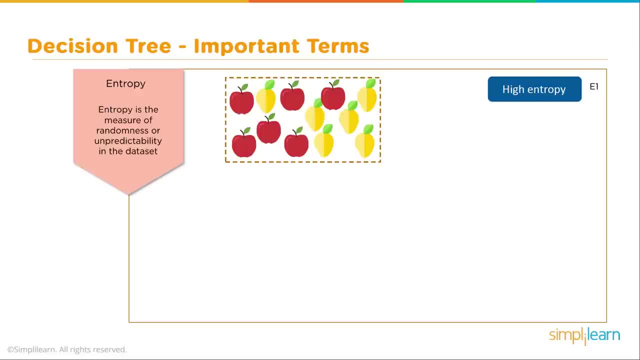 it wouldn't be able to tell you whether it's a lemon or an apple. It would just say it's a fruit. So the first thing we want to do is we want to split this apart And we take the initial data set and we're going to create a data set one and a data set two. 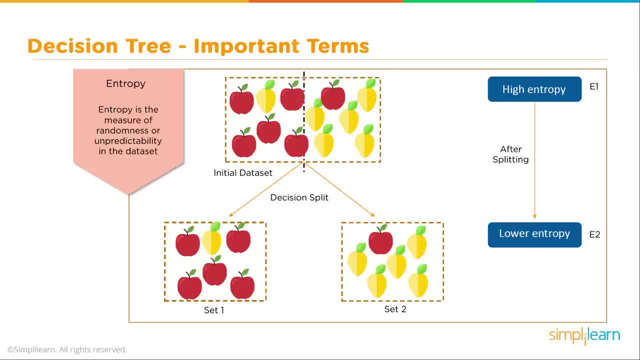 We just split it in two And if you look at these new data sets after splitting them, the entropy of each of those sets is much less. So for the first one, whatever comes in there, if this data goes this direction, it's probably an apple. 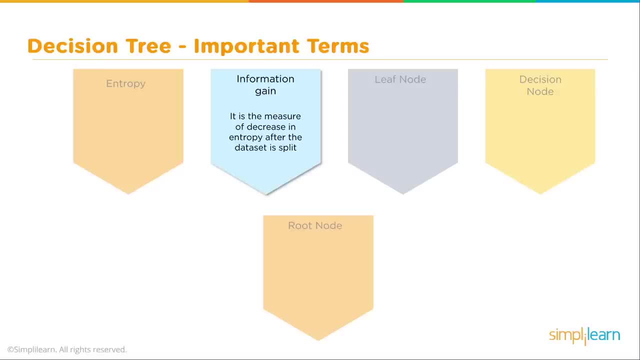 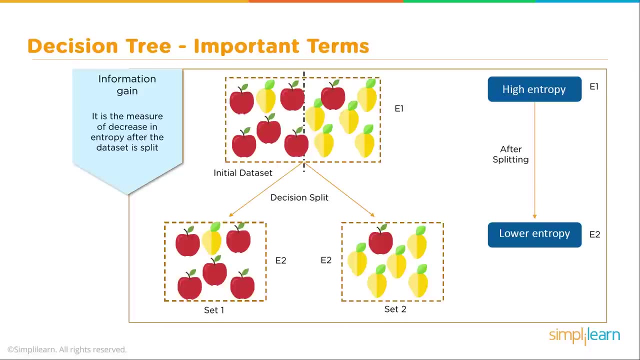 And if it goes into the other direction it's probably a lemon. So that brings us up to information gain. It is the measure of decrease in the entropy after the data set is split. What that means in here is that we've gone from one set. 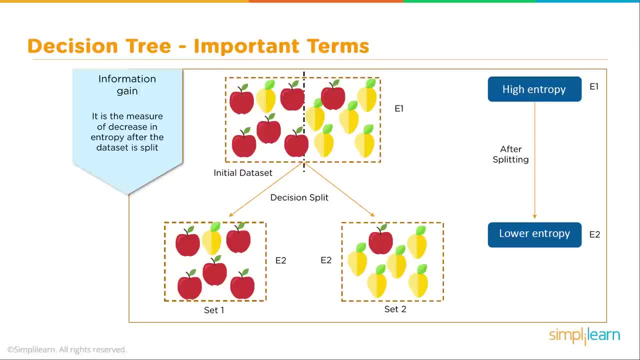 which has a very high entropy, to two lower sets of entropy, And we've added in the values of E1 for the first one and E2 for the second, two which are much lower, And so that information gain is increased greatly in this example. 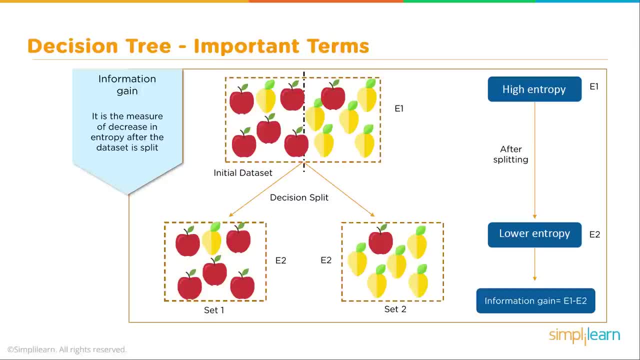 And so you can find that the information gain simply equals decision E1 minus E2.. As we're going down our list of definitions, we'll look at the leaf node, And the leaf node carries the classification or the decision. So we look down here to the leaf node. 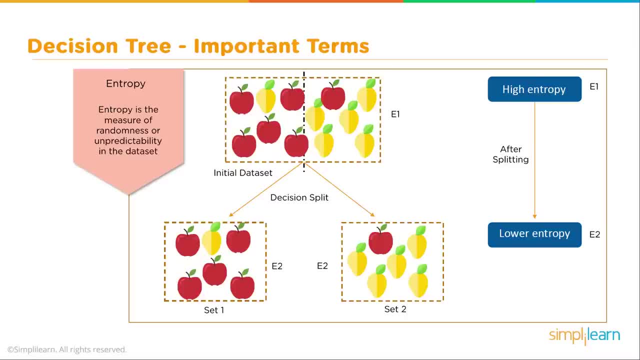 We finally get to our set one or our set two, When it comes down there and it says, okay, this object's gone into set one. if it's gone into set one, it's going to be split by some means, And we'll either end up with apples on the leaf node. 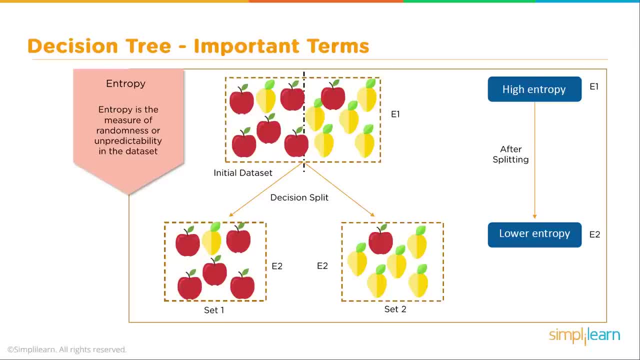 or a lemon on the leaf node, And on the right it'll either be an apple or lemons. Those leaf nodes are those final decisions or classifications. That's the definition of leaf node in here. If we're going to have a final leaf where we make the decision, 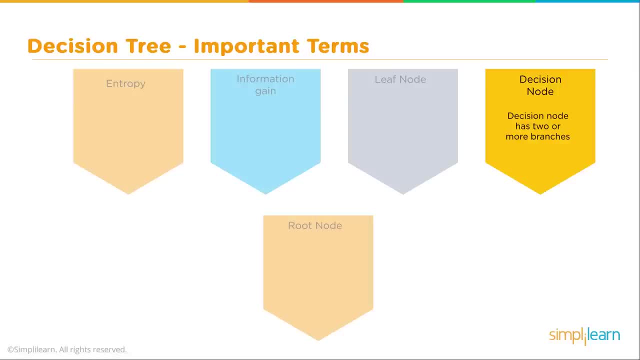 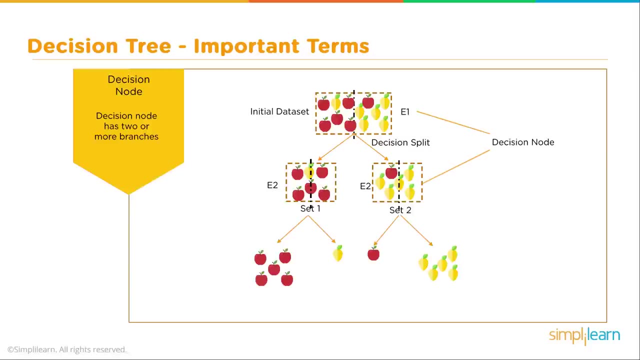 we should have a name for the nodes above it And they call those decision nodes A decision node. Decision node has two nodes, It has two or more branches And you can see here where we have the five apples and one lemon And in the other case the five lemons and one apple. 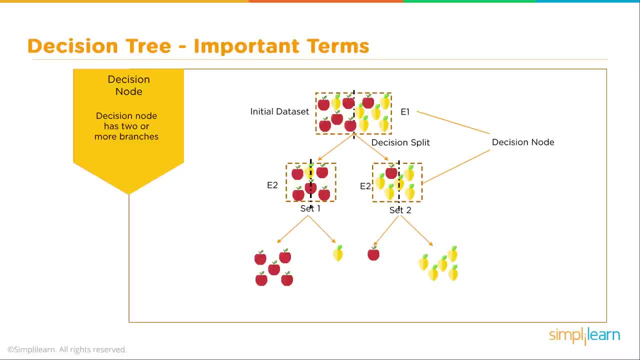 they have to make a choice of which tree it goes down, based on some kind of measurement or information given to the tree. And that brings us to our last definition, The root node. the topmost decision node is known as the root node. 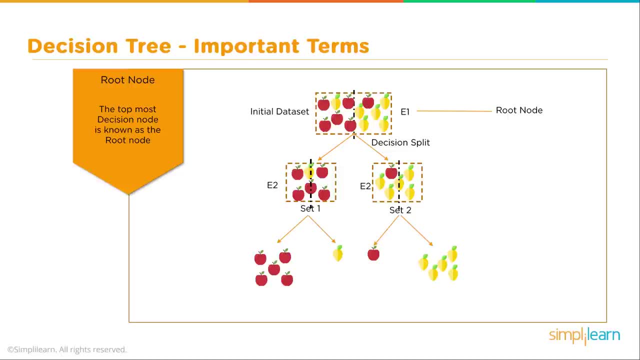 And this is where you have all of your data and you have your first decision. it has to make for split in information. So far we've looked at a very general image with the fruit being split. Let's look and see exactly what that means to split the data. 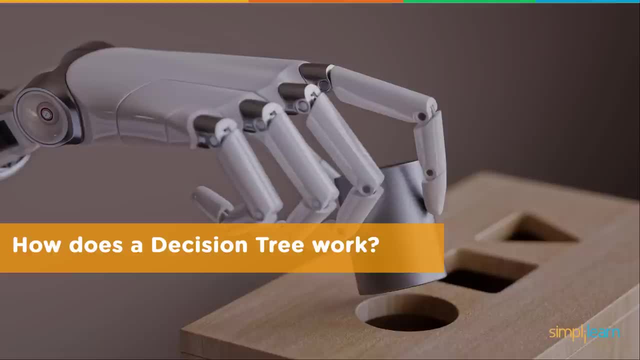 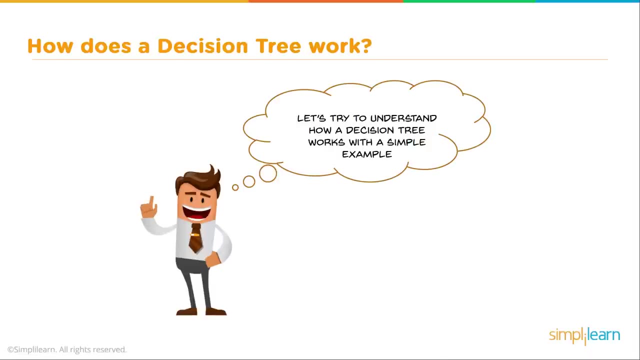 and how do we make those decisions on there? Let's go in there and find out how does a decision tree work. So let's try to understand this And let's use a simple example, And we'll stay with the fruit. We have a bowl of fruit. 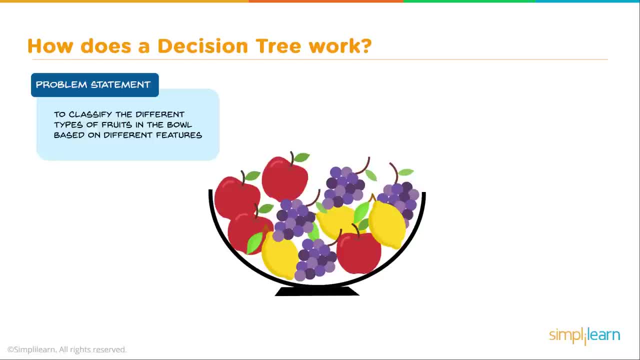 And so let's create a problem statement. And the problem is: we want to classify the different types of fruits in the bowl based on different features. The data set in the bowl is looking quite messy and the entropy is high in this case. So if this bowl was our decision maker? 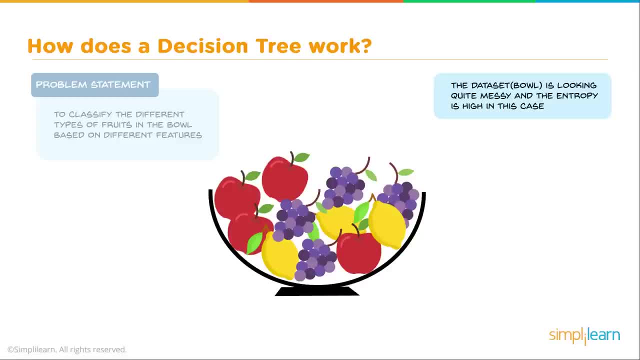 it wouldn't know what choice to make. It has so many choices. Which one do you pick? apple, grapes or lemons, And so we look in here We're going to start with a training set, So this is our data, that we're training our data with. 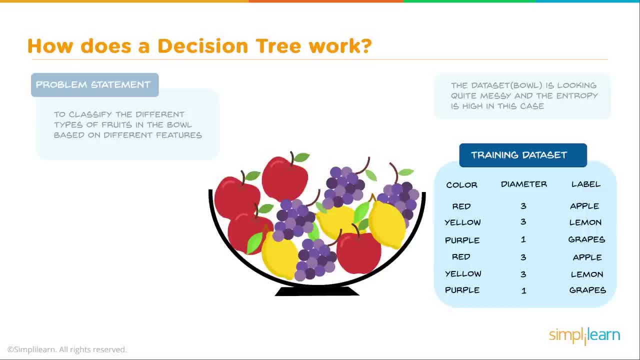 And we have a number of options here. We have the color And under the color we have red, yellow, purple. We have a diameter 3, 3, 1, 3, 3, 1.. And we have a label: apple lemon grapes. apple lemon grapes. 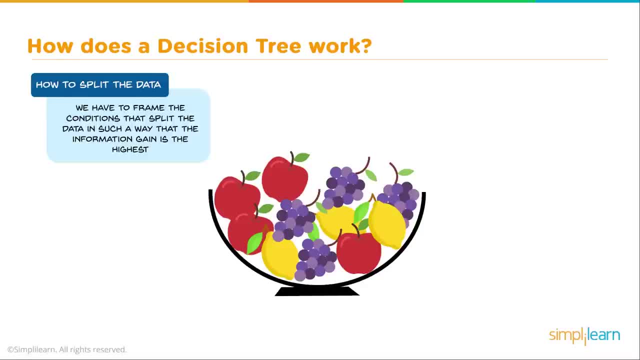 And how do we split the data? We have to frame the conditions to split the data in such a way that the information gain is the highest. It's very key to note that we're looking for the best gain. We don't want to just start sorting out the smallest piece in there. 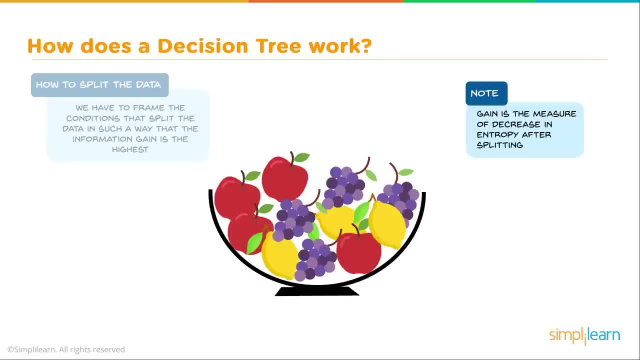 We want to split it the biggest way we can, And so we measure this decrease in entropy. That's what they call it- entropy After splitting, And now we'll try to choose a condition that gives us the highest gain. We will do that by splitting the data using each condition. 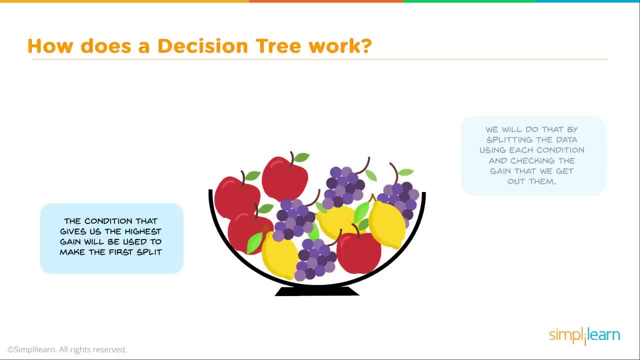 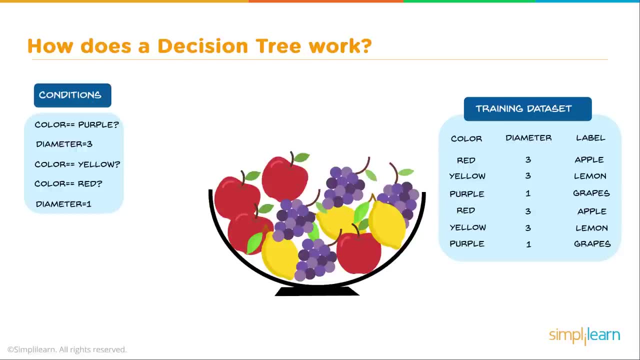 and checking the gain that we get out of them. The conditions that give us the highest gain will be used to make the first split. So let's take a look at these different conditions. We have color, We have diameter And if we look underneath that, we have a couple of different values. 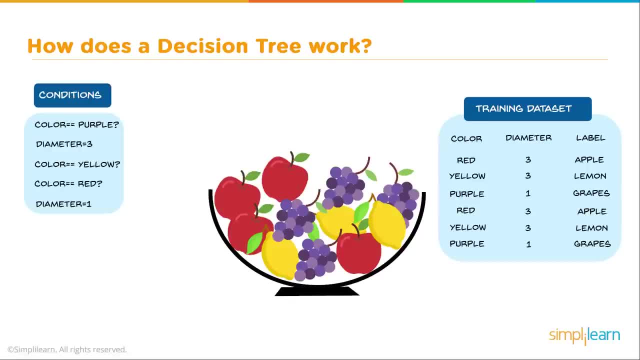 We have: diameter equals 3.. Color equals yellow, red. Diameter equals 1.. And when we look at that you'll see over here we have 1,, 2,, 3, 4, threes. That's a pretty hard selection. 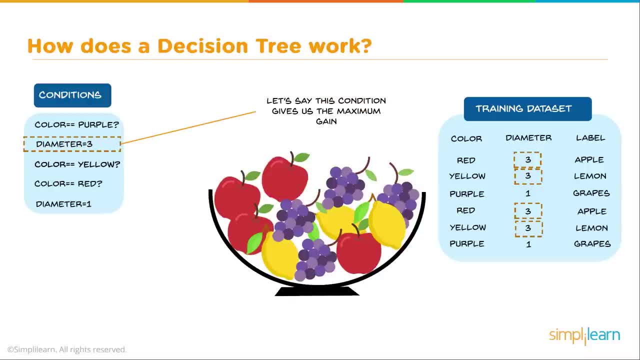 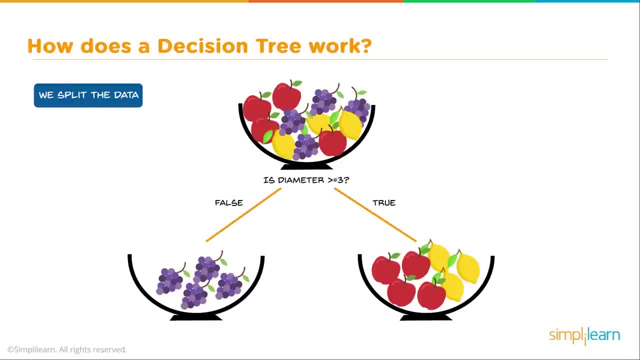 So let's say the condition gives us the maximum gain of 3.. So we have the most pieces fall into that range. So our first split from our decision node is we split the data based on the diameter. Is it greater than or equal to 3?? 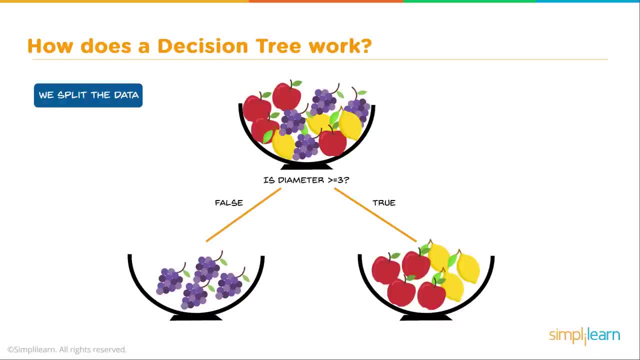 If it's not, that's false- It goes into the great bowl. And if it's true, it goes into the great bowl. And if it's true, it goes into the great bowl. It goes into a bowl full of lemon and apples. 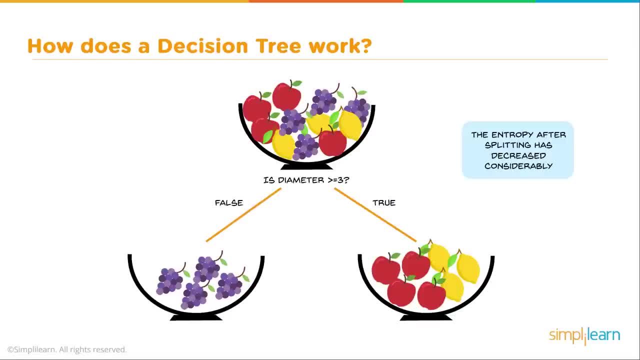 The entropy after splitting has decreased considerably, So now we can make two decisions. If you look, there's very much less chaos going on there. This node has already attained an entropy value of 0,. as you can see, There's only one kind of label left for this branch. 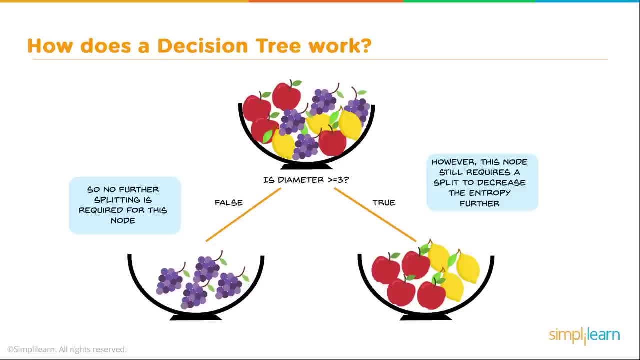 So no further splitting is required for this node. However, this node on the right still requires a split to decrease the entropy further. So we split the right node further based on the color. If you look at this, if I split it on color, that pretty much cuts it right down the middle. 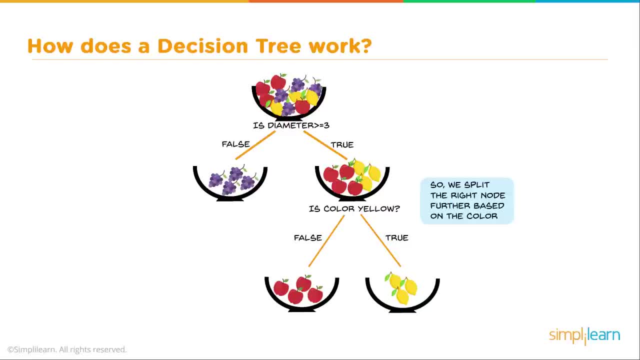 That's the only thing we have left in our choices of color and diameter too, And if the color is yellow, it's going to go to the right bowl, And if it's false, it's going to go to the left bowl. So the entropy in this case is now 0.. 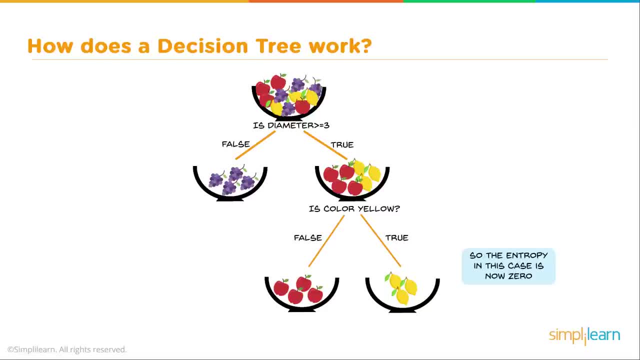 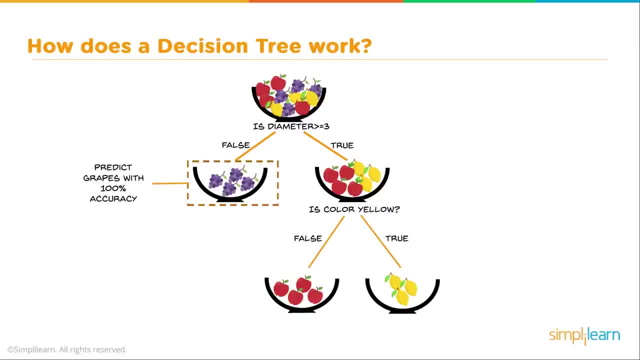 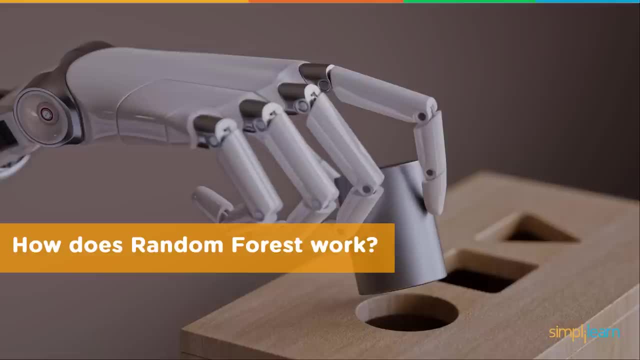 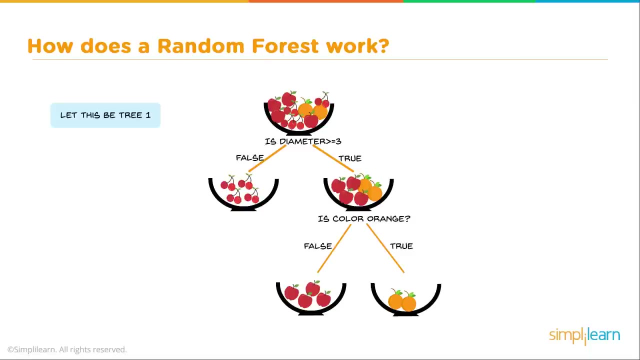 So we've looked at kind of a basic tree in our forest But what we really want to know is how does a random forest work as a whole? So to begin our random forest classifier, let's say we already have built three trees And we're going to start with the first tree that looks like this: 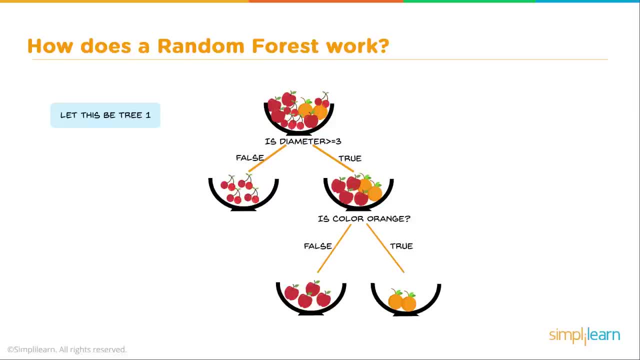 Just like we did in the example. this tree looks at the diameter. If it's greater than or equal to 3, it's true. Otherwise it's false. So one side goes to the smaller tree. Smaller diameter: One side goes to the larger diameter. 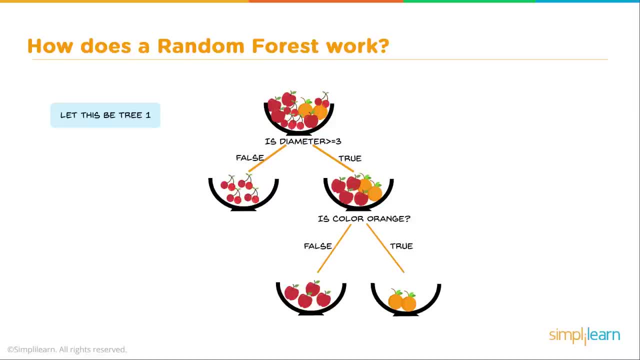 And if the color is orange, it's going to go to the right. True, We're using oranges now instead of lemons. And if it's red, it's going to go to the left. False, We build a second tree. 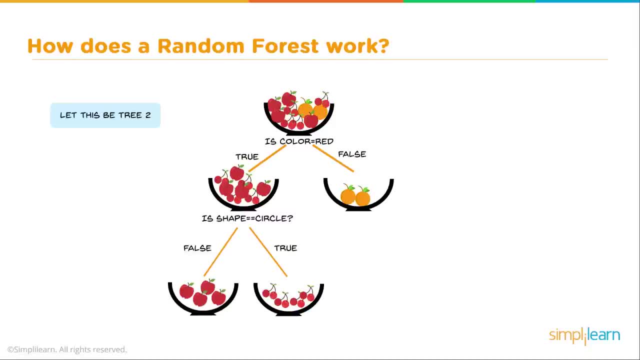 Very similar, But it's split differently. Instead of the first one being split by a diameter, this one. when they created it. if you look at that first bowl, it has a lot of red objects. So it says: is the color red? 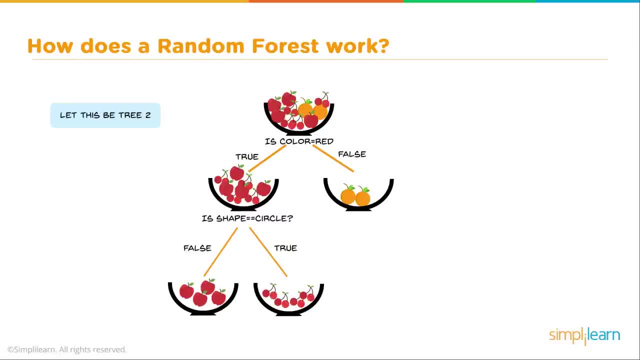 Because that's going to bring our entropy down the fastest. And so, of course, if it's true, it goes to 3.. If it's true, it goes to the left. If it's false, it goes to the right. 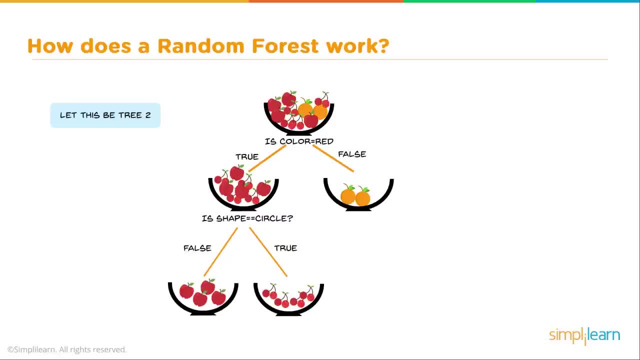 And then it looks at the shape: false or true, and so on and so on. And tree 3,: is the diameter equal to 1?? And it came up with this because there's a lot of cherries in this bowl, So that would be the biggest split on there is. is the diameter equal to 1?? 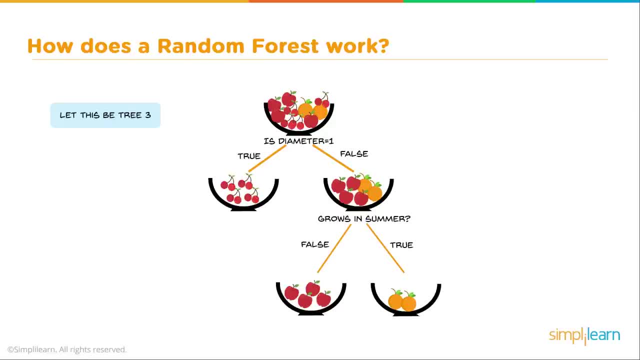 That's going to drop the entropy the quickest And, as you can see, it splits it into true. If it goes false- and they've added another category- does it grow in the summer? And if it's false, it goes off to the left. 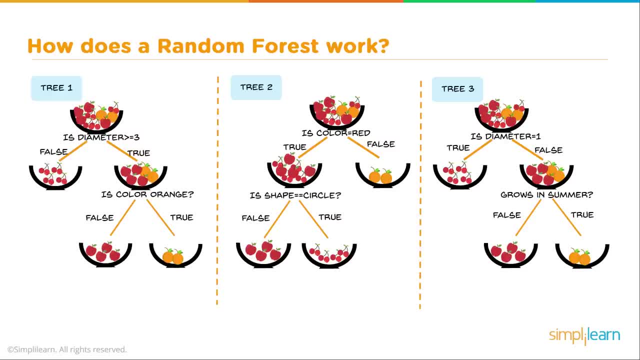 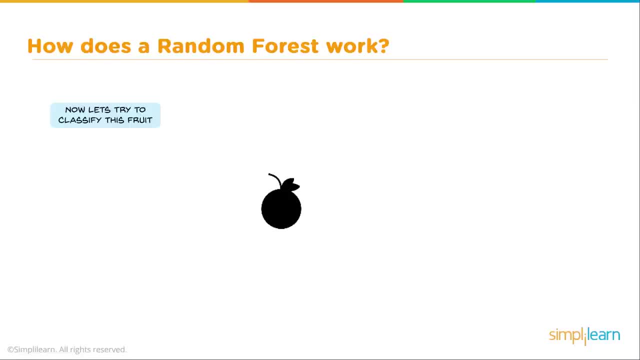 If it's true, it goes off to the right. Let's go ahead and bring these three trees. You can see them all in one image. So this would be three completely different trees categorizing a fruit, And let's take a fruit. 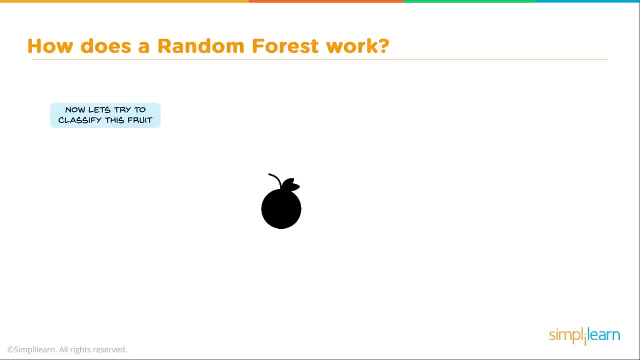 Now let's try this And this fruit. if you look at it, we've blackened it out. You can't see the color on it, So it's missing data. Remember, one of the things we talked about earlier is that a random forest works really. 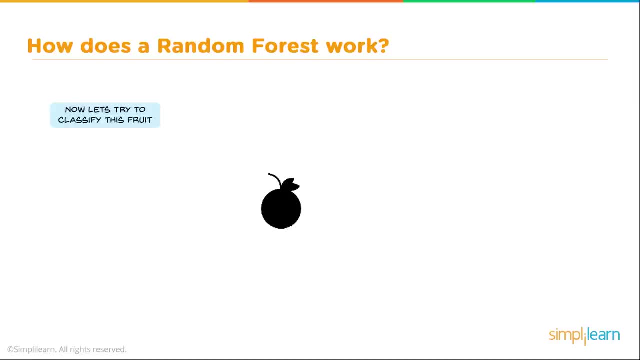 good if you're missing data, if you're missing pieces. So this fruit has an image, but maybe the person had a black and white camera when they took the picture And we're going to take a look at this And it's going to have they put the color in there. 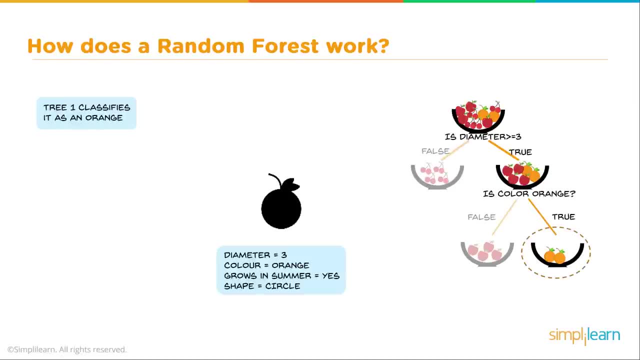 So ignore the color down there. But the diameter equals three, We find out it grows in the summer. equals yes, And the shape is a circle. And if you go to the right you can look at what one of the decision trees did. 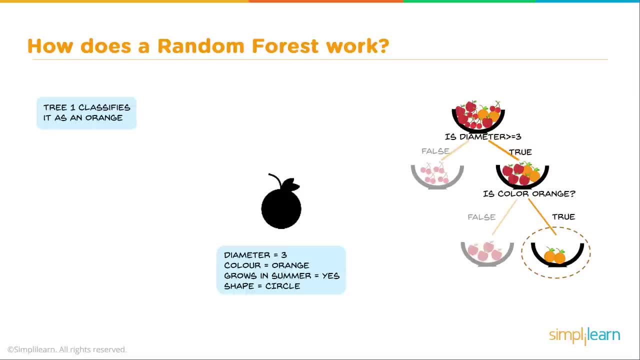 This is the third one: Is the diameter greater than equal to three? Is the color orange? Well, it doesn't really know on this one, But if you look at the value, it'd say true and it'd go to the right. 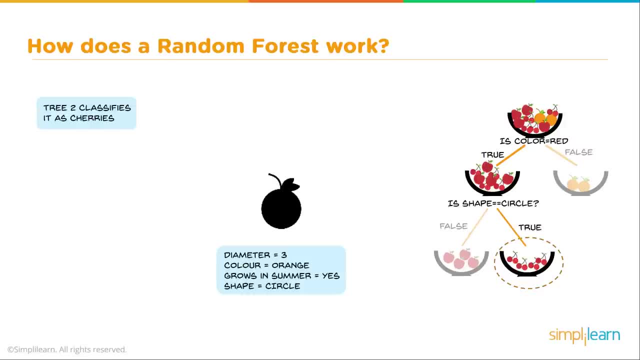 Tree. two classifies it as cherries. Is the color equal- red. Is the shape: a circle? True, it is a circle. So this would look at it and say, oh, that's a cherry. And then we go to the other classifier and it says: is the diameter equal one? 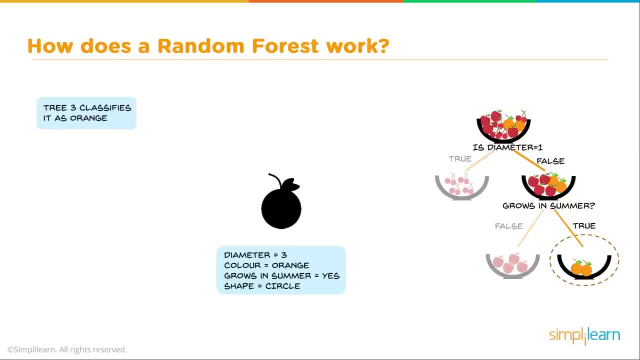 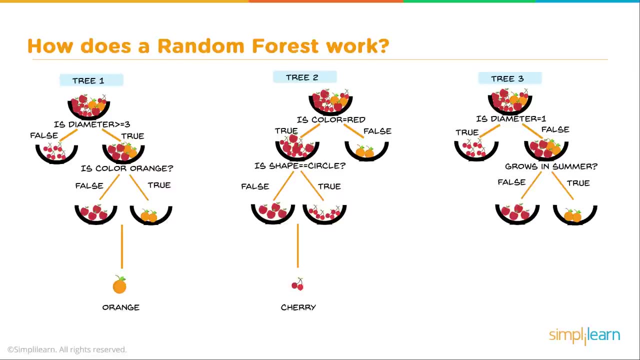 Well, that's false. Does it grow in the summer? True, So it goes down and looks at as oranges. So how does this random forest work? The first one says it's an orange, The second one said it was a cherry. 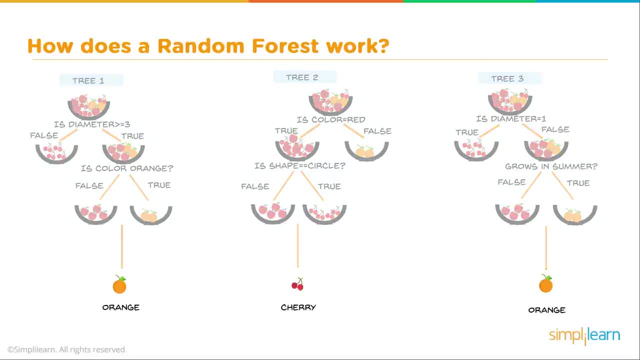 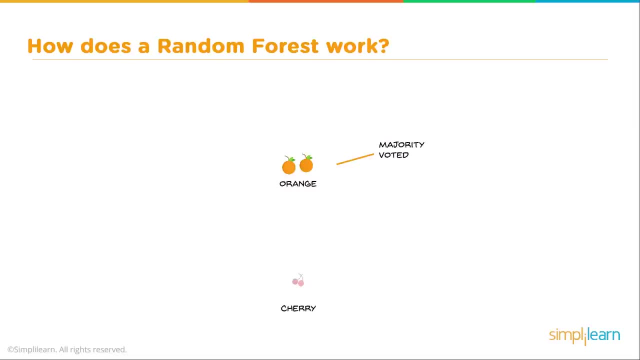 And the third one says it's an orange, And you can guess if you have two oranges and one says it's a cherry. when you add that all together, the majority of the vote says orange. So the answer is it's classified as an orange even though we didn't know the color and we're 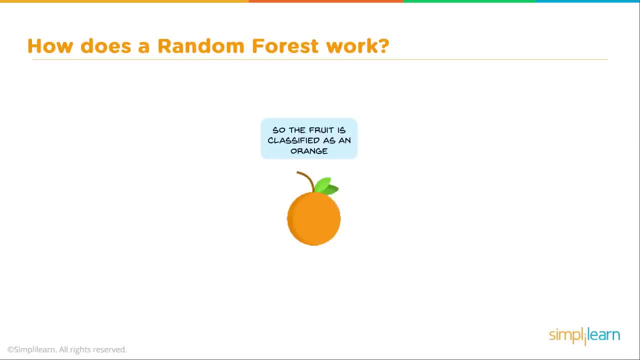 missing data on it. I don't know about you, but I'm getting tired of fruit, So let's switch. And I did promise you we'd start looking at a case example and get into some Python coding. Today we're going to use the case: the iris flower analysis. 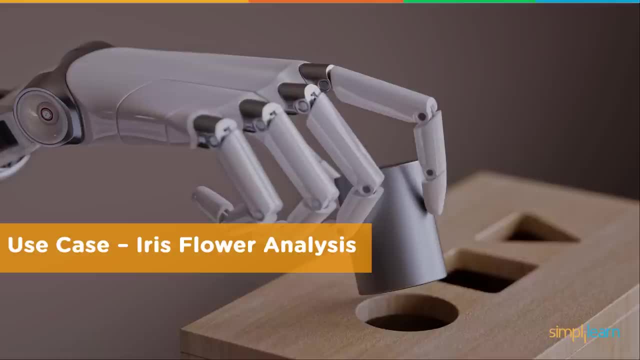 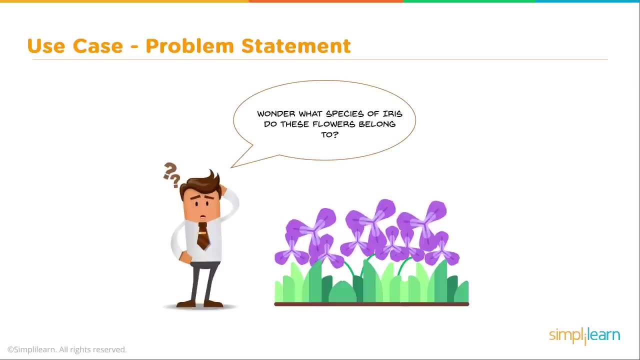 This is the exciting part, as we roll up our sleeves and actually look at some Python coding. Before we start the Python coding, we need to go ahead and create a problem statement: Wonder: what species of iris do these flowers belong to? Let's try to predict the species of the flowers using machine learning in Python. 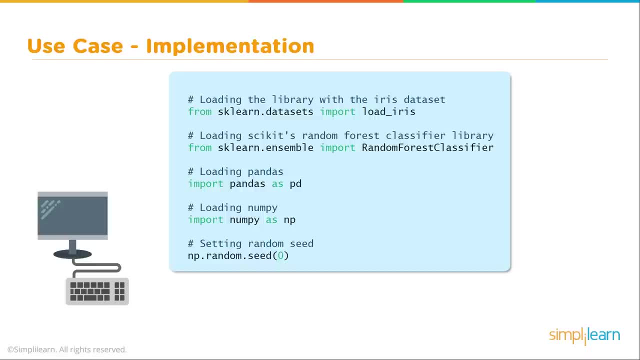 Let's see how it can be done. So here we begin to go ahead and implement our Python code, And you'll find that the first half of our implementation is all about organizing and exploring the data coming in. Let's go ahead and take this first step, which is loading the different modules into Python. 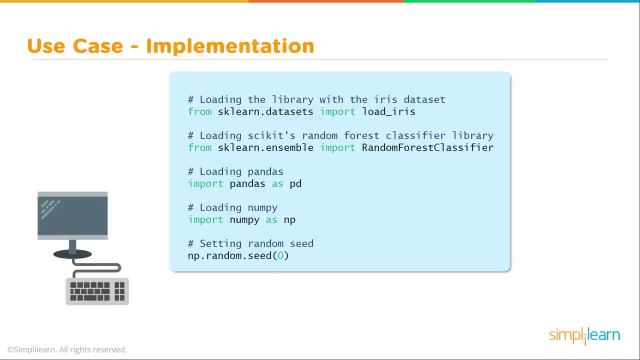 And let's go ahead and put that in our favorite editor. whatever your favorite editor is, In this case I'm going to be using the Anaconda Jupyter Notebook, which is one of my favorites. Certainly, there's Notepad++ and Eclipse and dozens of others. 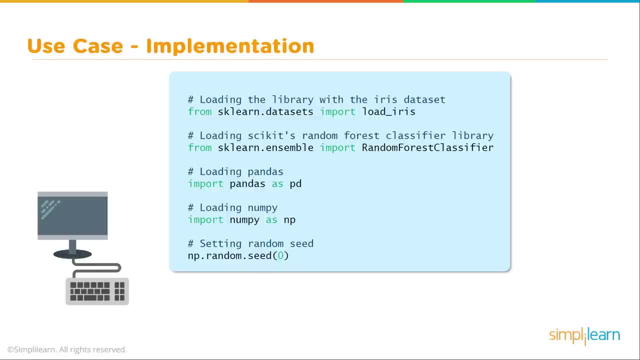 or just even using the Python terminal window- Any of those will work just fine to go ahead and explore this Python coding. So here we go. Let's go ahead and flip over to our Jupyter Notebook, And I've already opened up a new page for Python 3 code. 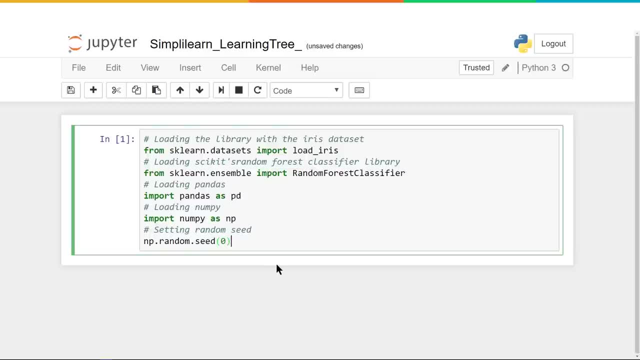 And I'm just going to paste this right in there. So let's go ahead and click on that link And let's go ahead and take a look and see what we're bringing into our Python. The first thing we're going to do is, from the sklearndatasets, import loadiris. 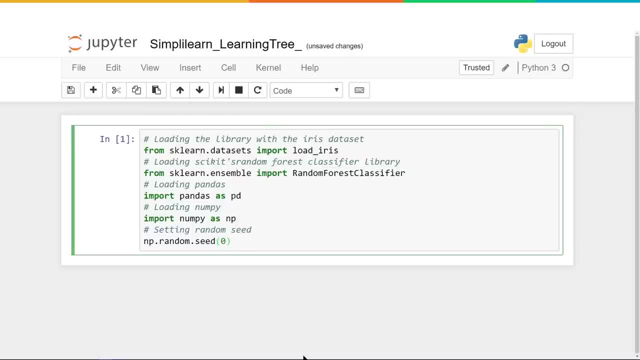 Now, this isn't the actual data. this is just the module that allows us to bring in the data. the loadiris And the iris is so popular. it's been around since 1936, when Ronald Fisher published a paper on it. 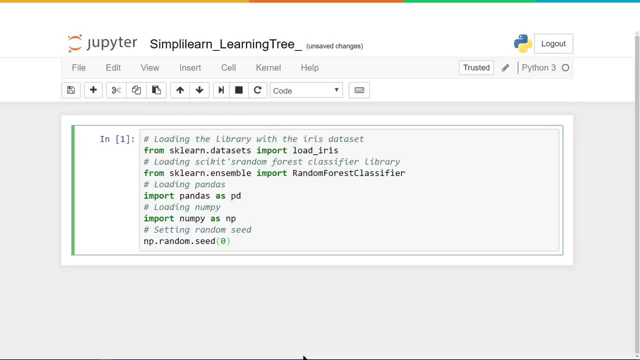 And they're measuring the different parts of the flower And, based on those measurements, predicting what kind of flower it is. And then, if we're going to do a random forest classifier- we're going to do this- We need to go ahead and import a random forest classifier from the sklearn module. 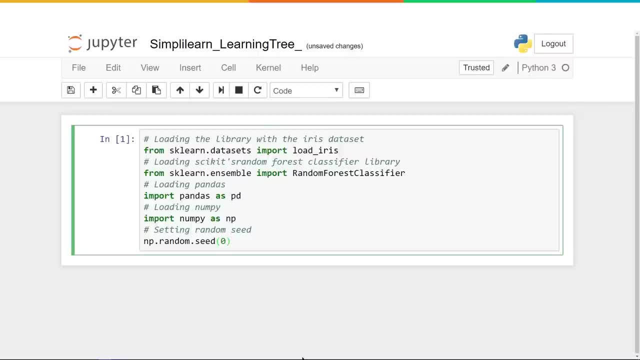 So sklearnensemble, import random forest classifier. And then we want to bring in two more modules, And these are probably the most commonly used modules in Python and data science with any of the other modules that we bring in- And one is going to be pandas- 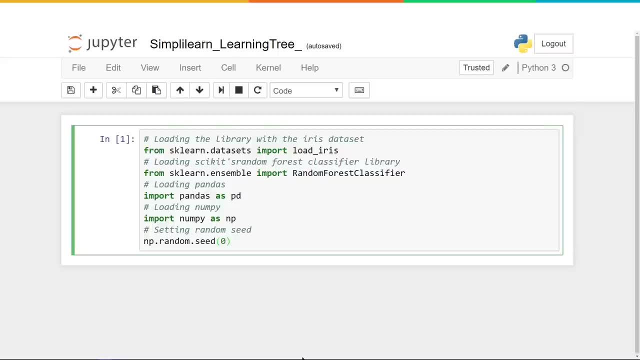 We're going to import pandas as pd. pd is a common term used for pandas And pandas basically creates a data format for us where, when you create a pandas data frame, it looks like an XSKL spreadsheet, And you'll see that in a minute when we start digging deeper into the code. 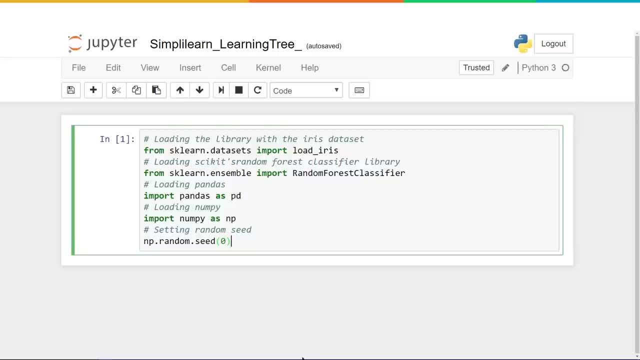 Pandas is just wonderful because it plays nice with all the other modules in there. And then we have numpy, which is our numbers Python, And the numbers Python allows us to do different mathematical sets on here. We'll see right off the bat we're going to take our np. 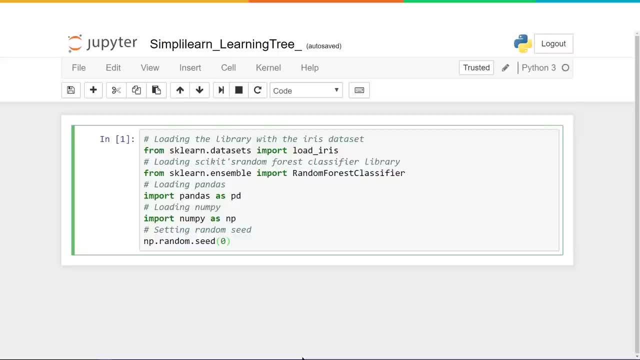 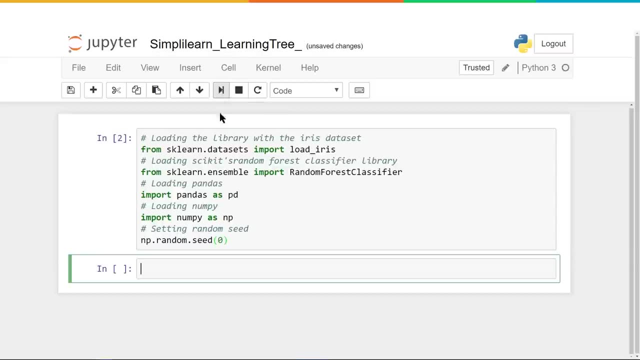 and we're going to go ahead and seed the range Randomness with. it was zero, So nprandomseed is seeding that as zero. This code doesn't actually show anything. We're going to go ahead and run it because I need to make sure I have all those loaded. 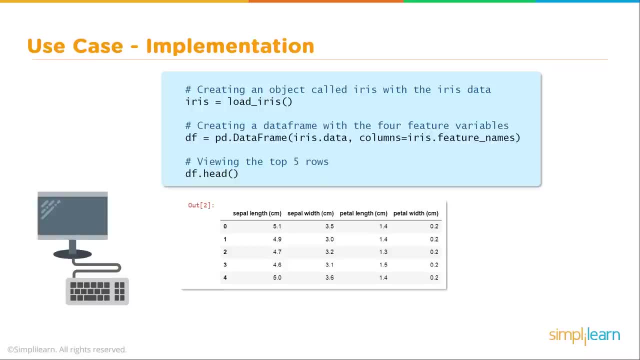 And then let's take a look at the next module on here. The next six slides, including this one, are all about exploring the data. Remember, I told you half of this is about looking at the data and getting it all set. So let's go ahead and take this code right here: the script. 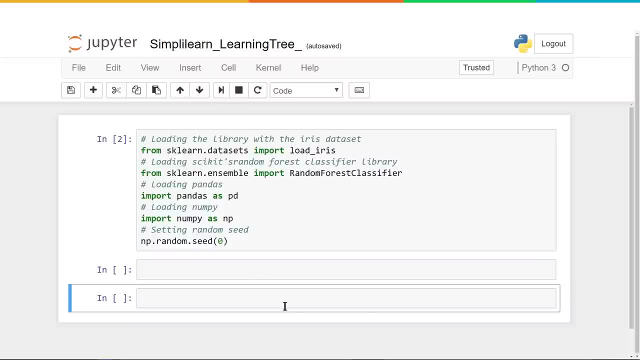 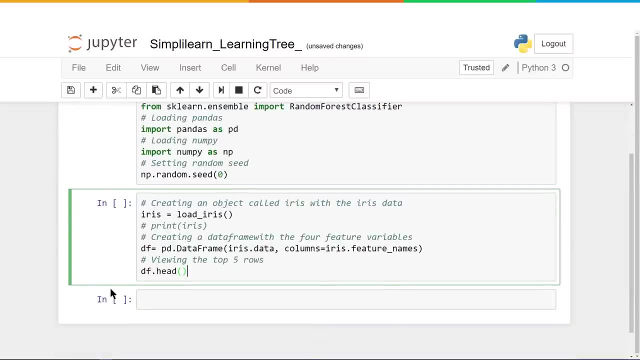 and let's get that over into our Jupyter notebook And here we go. We've gone ahead and run, I'm going to run the imports and I'm going to paste the code down here And let's take a look and see what's going on. 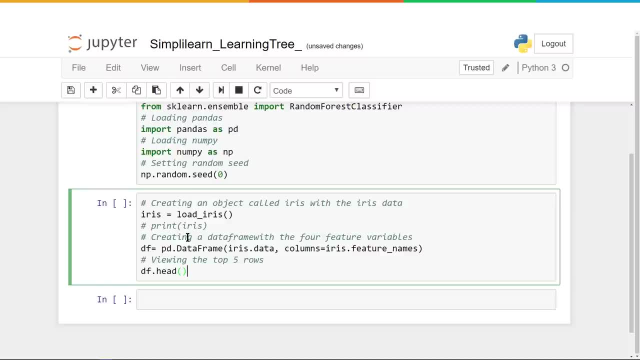 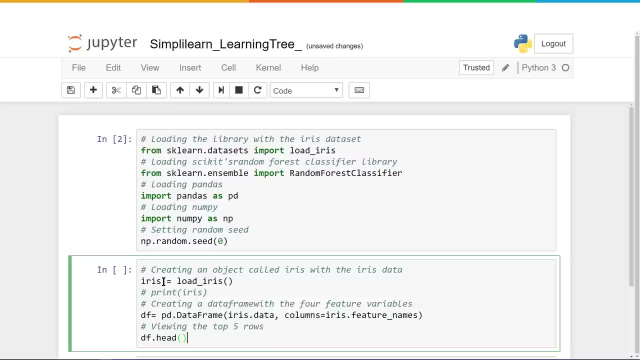 The first thing we're doing is we're actually loading the iris data And, if you remember, up here we loaded the module that tells it how to get the iris data. Now we're actually assigning that data to the variable iris And then we're going to go ahead and use the df to define data frame. 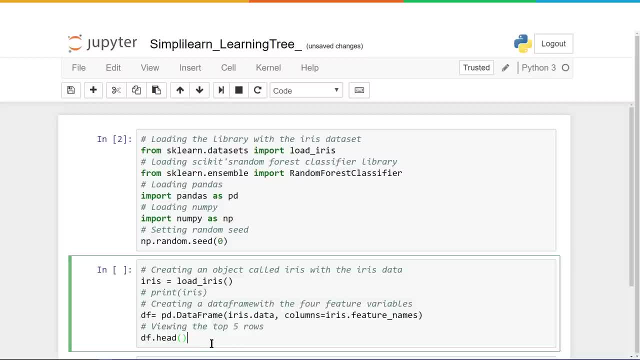 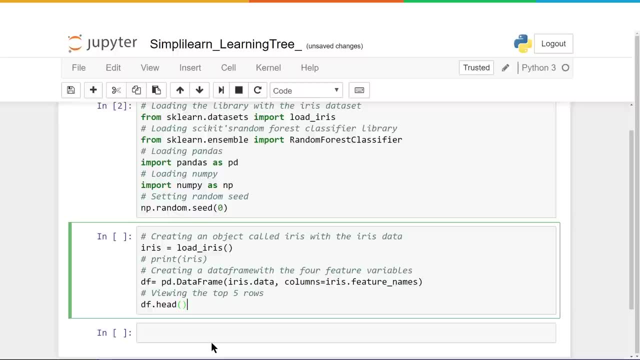 And that's going to equal pd And if you remember, that's pandas as pd. So that's our pandas And panda data frame. And then we're looking at iris data and columns equals iris feature names And we're going to do the df head. 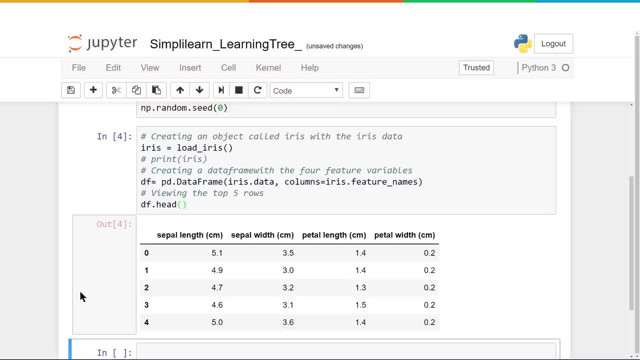 And let's run this so you can understand what's going on here. The first thing you want to notice is that our df has created what looks like an Excel spreadsheet And in this Excel spreadsheet we have set the columns, So up on the top you can see the four different columns. 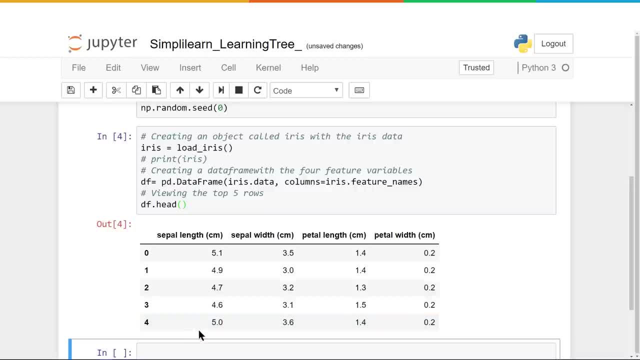 And then we have the data- irisdata- down below. It's a little confusing Without knowing where this data is coming from. So let's look at the bigger picture And I'm going to go print. I'm just going to change this for a moment. 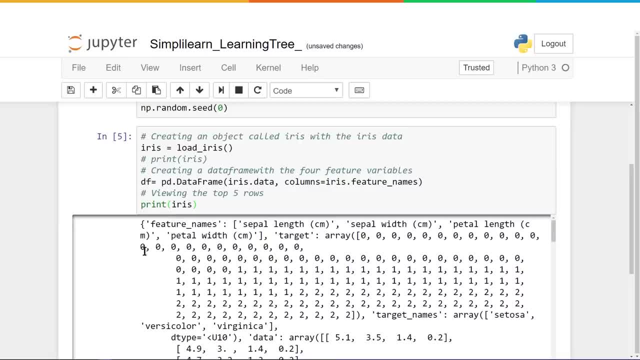 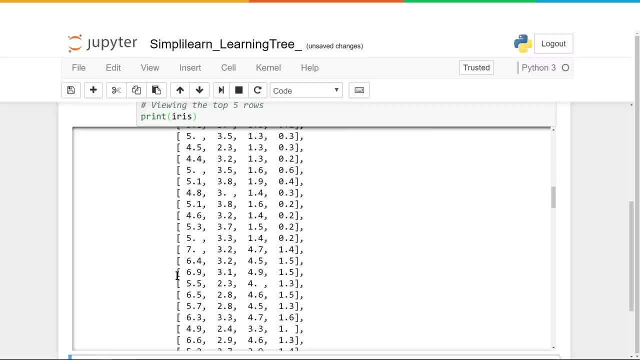 And we're going to print all of iris And see what that looks like. So when I print all of iris, I get this long list of information And you can scroll through here and see all the different titles on there. What's important to notice is that, first off, there's brackets at the beginning. 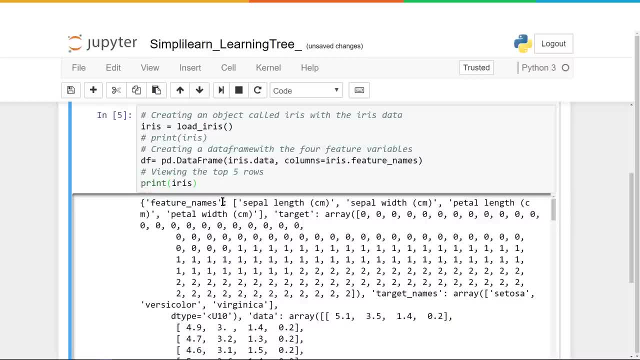 So this is a Python dictionary, And in a Python dictionary you'll have a key or a label and this label pulls up whatever information comes after it. So feature names which we actually used over here under columns- is equal to an array of sepal length, sepal width. petal length, petal width. 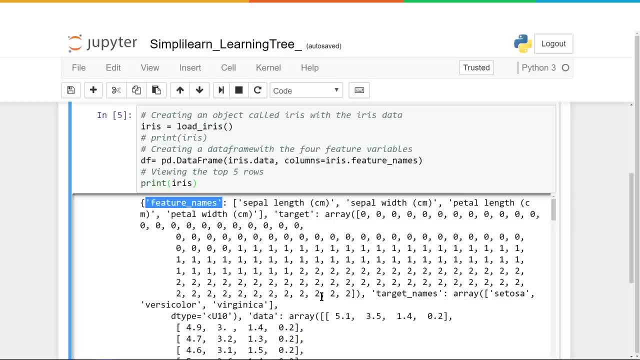 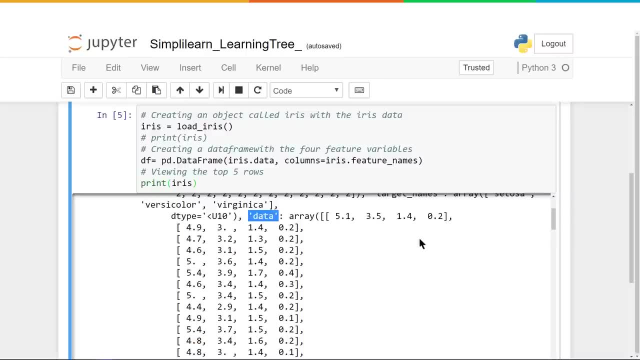 These are the different names they have for the four different columns And if you scroll down far enough, you'll also see data down here. Oh goodness, it came up right towards the top And data is equal to the different data we're looking at. 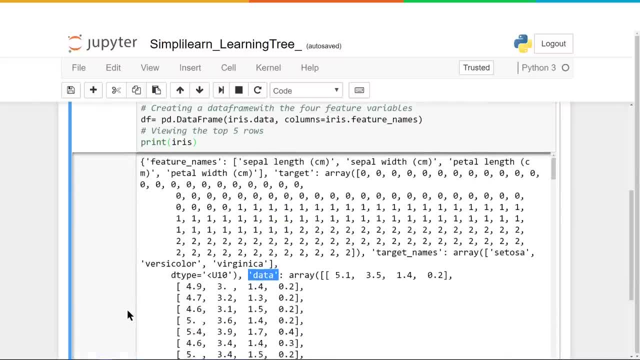 Now there's a lot of other things in here, like target- We're going to be pulling that up in a minute- And there's also the names, the target names, which is further down, And we'll show you that also in a minute. 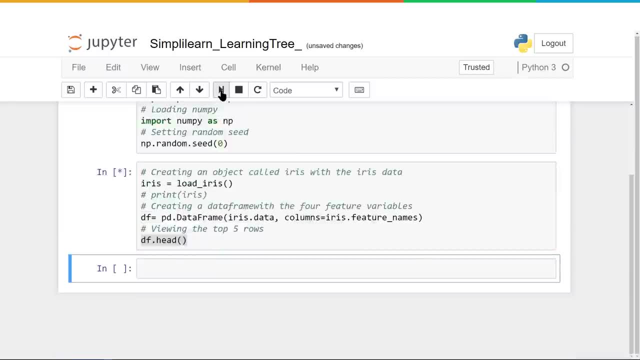 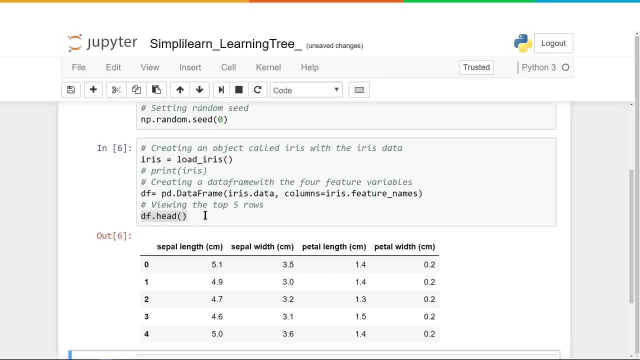 Let's go ahead and set that back to the head. And this is one of the neat features of pandas and panda data frames Is, when you do dfhead or the panda data framehead, it'll print the first five lines of the data set in there. Along with the headers, if you have it. In this case, we have the data set And we're going to print the first five lines of the data set in there Along with the headers, if you have it. In this case, we have the data set. 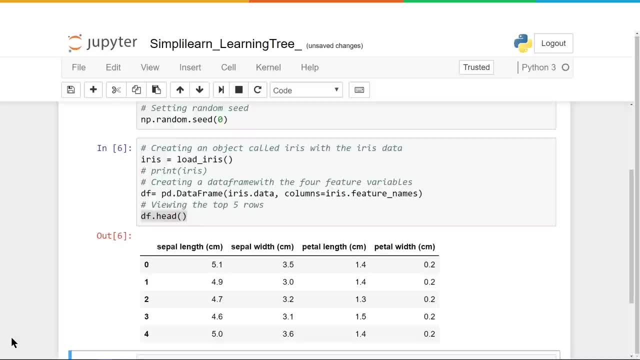 And we have the column headers set to iris features And in here you'll see that we have 0, 1,, 2, 3, 4.. In Python, most arrays always start at 0.. So when you look at the first five, it's going to be 0, 1, 2, 3, 4, not 1, 2, 3, 4, 5.. 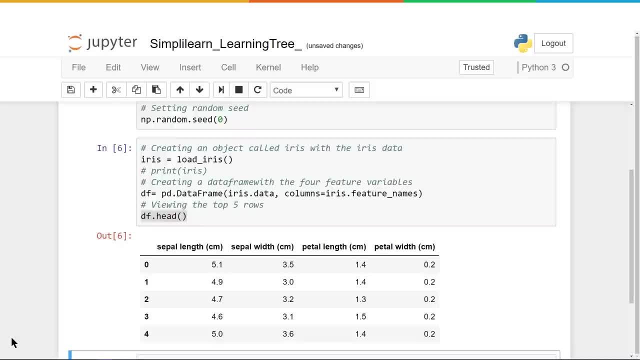 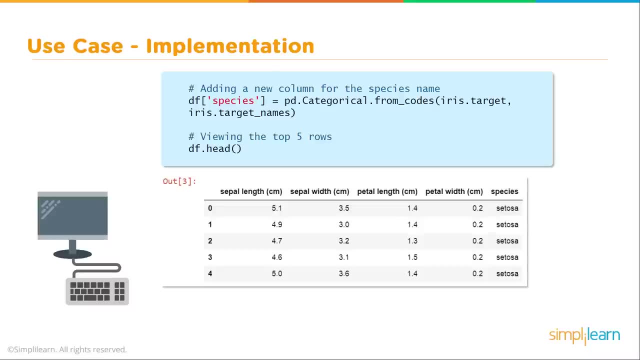 So now we've got our iris data imported into a data frame, Let's take a look at the next piece of code in here. And so in this section here of the code, we're going to take a look at the target And let's go ahead and get this into our notebook, this piece of code. 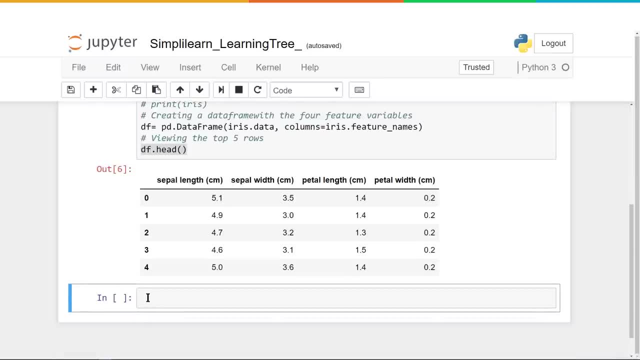 So we can see that we have the data set in there. So we can discuss it a little bit more in detail. So here we are in our Jupyter notebook. I'm going to put the code in here And before I run it I want to look at a couple things going on. 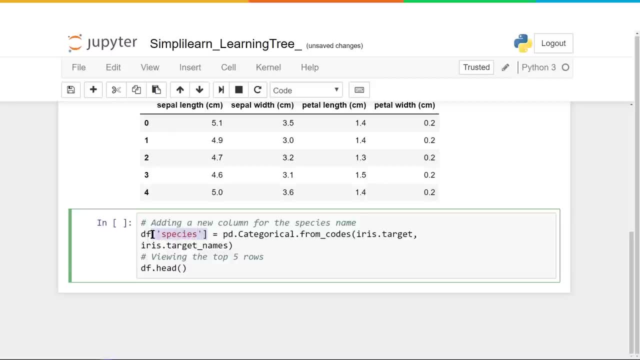 So we have df species, And this is interesting because right here you'll see where I have df species in brackets, which is the key code for creating another column, And here we have iristarget. Now these are both in the pandas setup on here. 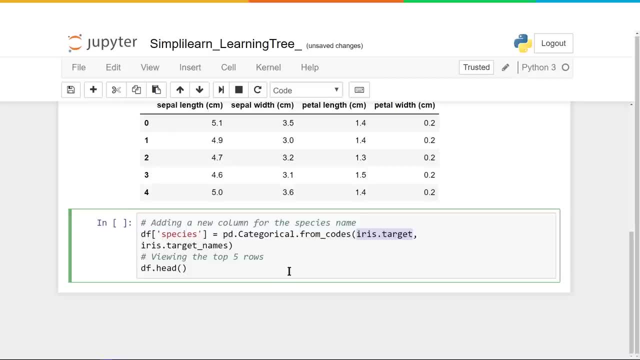 So in pandas we can do either one. I could have just as easily done iris and then in brackets, target, depending on what I'm working on, Both are acceptable. Let's go ahead and run this code and see how this changes. 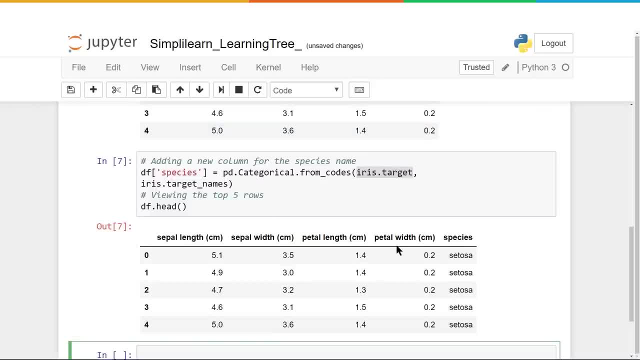 And what we've done is we've added the target from the iris data set as another column on the end. Now, what species is? this is what we're trying to predict. So we have our data, which tells us the answer for all these different pieces. 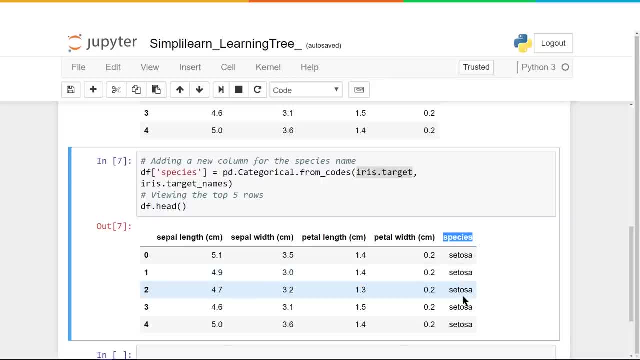 And then we've added a column with the answer. That way, when we do our final setup will have the ability to program our neural network to look for these, this different data, and know what a setosa is, or a vericolor- which we'll see in just a minute- or virginica. 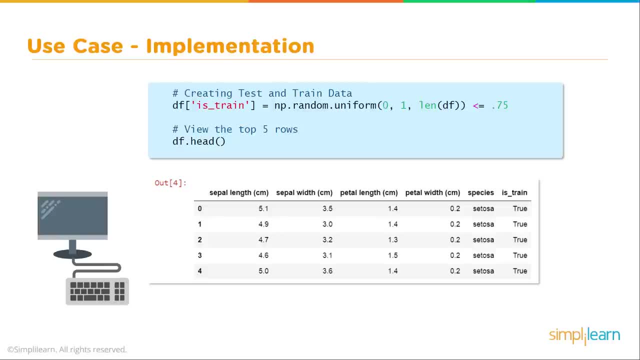 Those are the three that are in there, And now we're going to add one more column. I know we're organizing all this data over and over again. It's kind of fun. There's a lot of ways to organize it. What's nice about putting everything onto one data frame is I can then do a printout and it shows me exactly what I'm looking at. 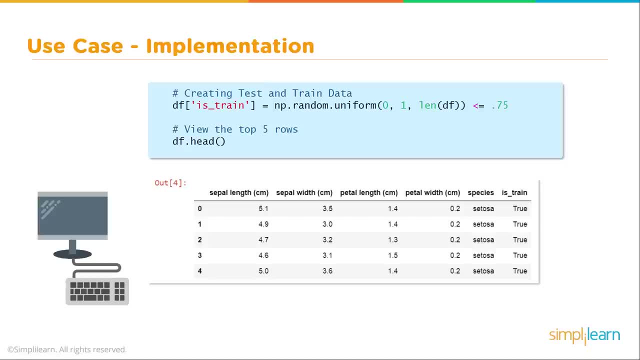 And I'll show you how to do that in just a minute. And I'll show you how to do that in just a minute And I'll show you where that's different, where you can alter that and do it slightly differently. But let's go ahead and put this into our script. up to that now. 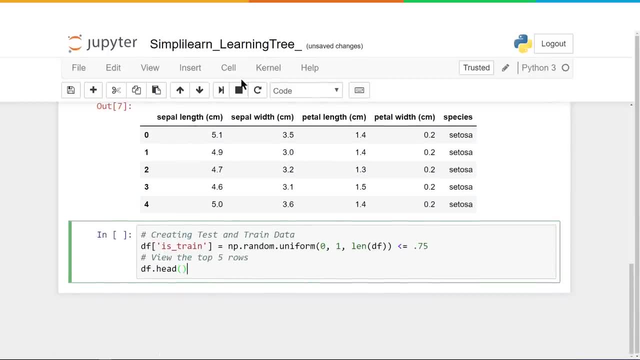 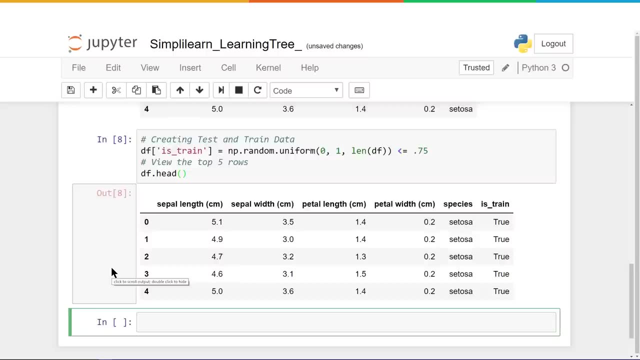 And here we go. We're going to put that down here and we're going to run that, And let's talk a little bit about what we're doing Now. we're exploring data And one of the challenges is knowing how good your model is. 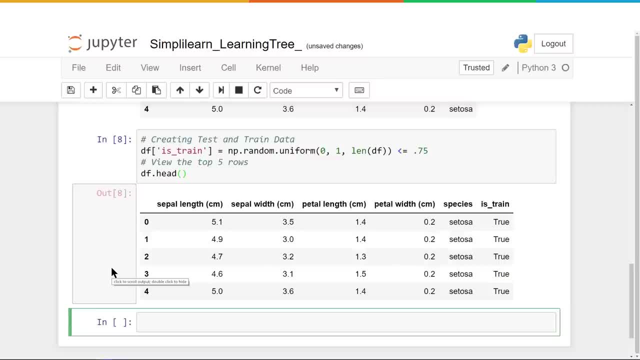 Did your model work, And to do this we need to split the data, and we split it into two different parts. They usually call it the training And the testing, And so in here we're going to go ahead and put that in our database so you can see it clearly. 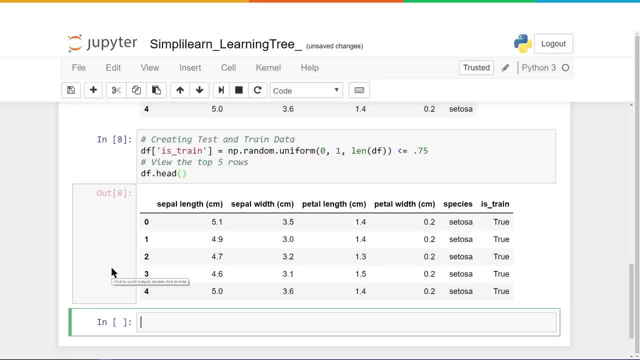 And we've set it df And remember you can put brackets. This is creating another column Is train, So we're going to use part of it for training. And this equals np. Remember that stands for numpy, randomuniform, So we're generating a random number between 0 and 1.. 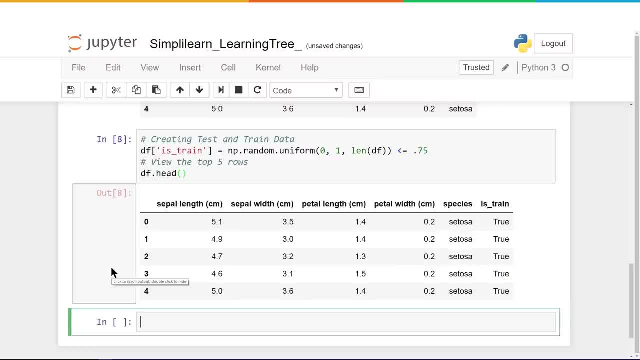 And we're going to do it for each of the rows. That's where the length df comes from. So each row gets a generated number, And if it's less than 0.75, it's true, And if it's greater than 0.75, it's false. 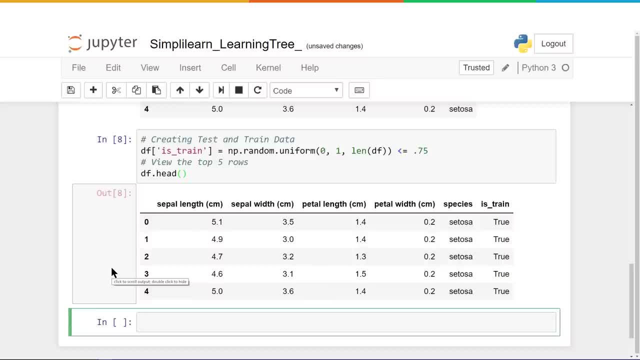 This means we're going to take 75% of the data roughly, because there's a randomness involved And we're going to use that to train it, And then the other 25% we're going to hold off to the side and use that to test it later on. 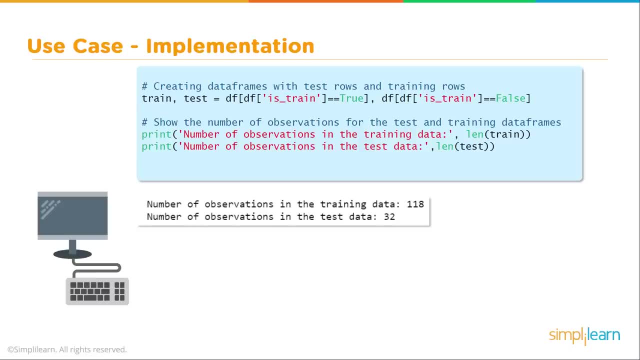 So let's flip back out over and see what the next step is. So, now that we've labeled our database for which is training and which is testing, let's go ahead and sort that into two different variables- Train and testing- And let's take this code and let's bring it into our project. 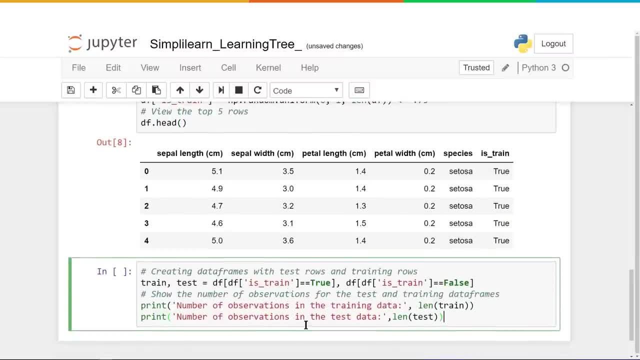 And here we go. Let's paste it on down here. And before I run this, let's just take a quick look at what's going on here. What we're going to do here is we have up above, we created. remember there's our defhead. 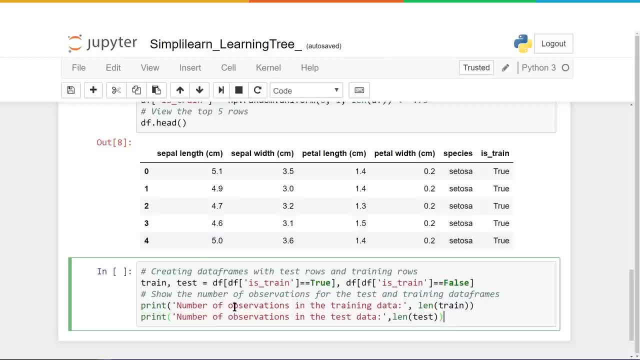 which prints the first five rows, And we've added a column, is train at the end. And so we're going to take that and we're going to create two variables. We're going to create two new data frames. One's called train. 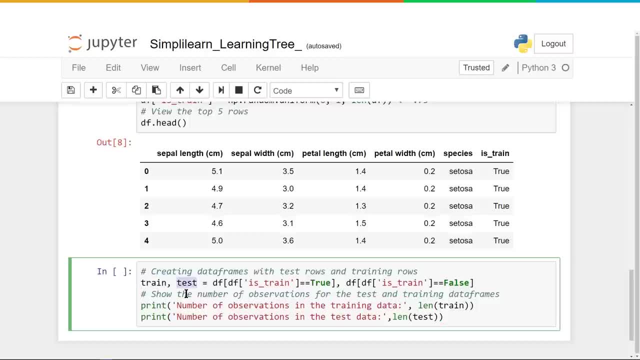 One's called test, 75% in train, 25% in test. And then to sort that out, we're going to do that by doing df, our original data frame, with the iris data in it. And if df is train equals, true, that's going to go in the train. 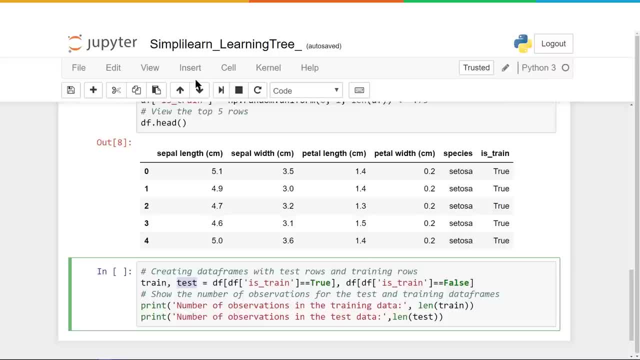 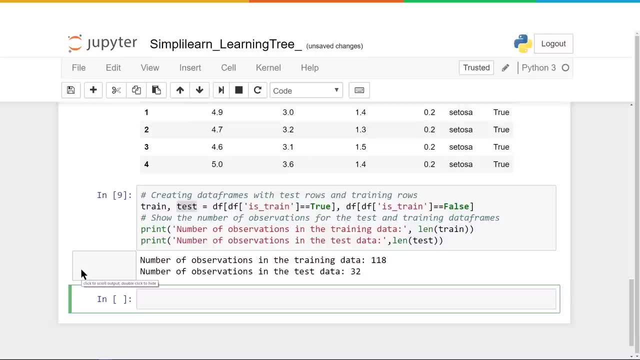 And if df is train equals false, it goes in the test, And so when I run this, we're going to print out the number in each one. Let's see what that looks like And you'll see that it puts 118 in the training module. 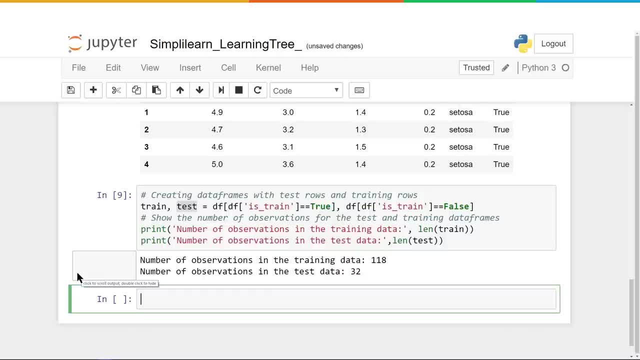 And it puts 32 in the testing module, which lets us know that there was 150 lines of data in here. So if you went and looked at the original data, you could see that there's 150 lines And that's roughly 75% in one and 25% for us to test our model on afterward. 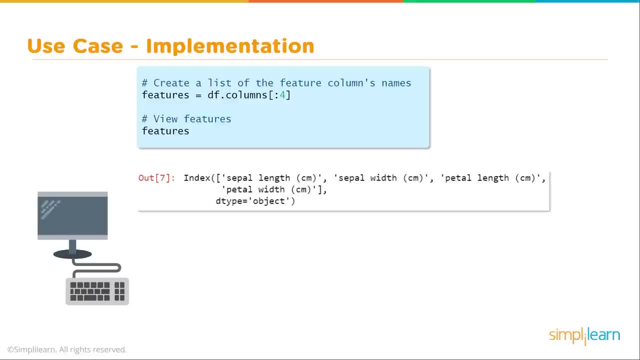 So let's jump back to our code and see where this goes. In the next two steps, we want to do one more thing with our data, And that's make it readable to humans. I don't know about you, but I hate looking at zeros and ones. 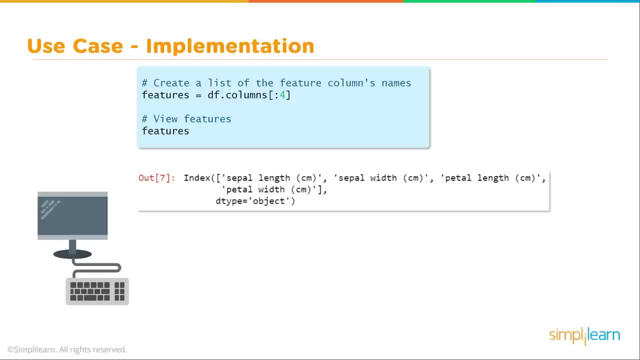 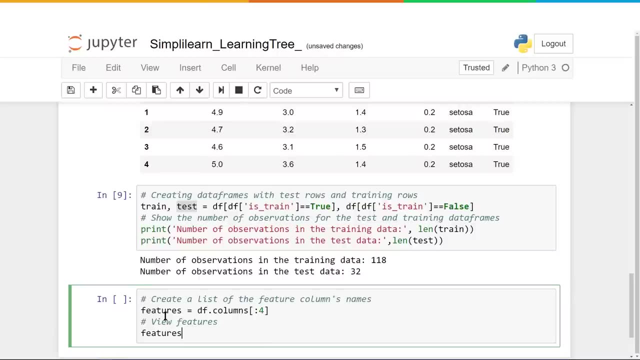 So let's start with the features And let's go ahead And take those and make those readable to humans And let's put that in our code. Let's see, Here we go, Paste it in And you'll see, here we've done a couple very basic things. 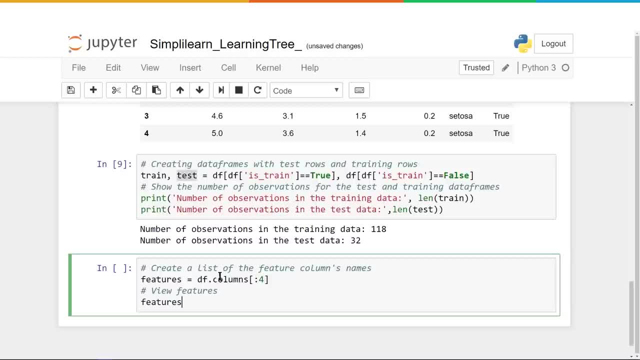 We know that the columns in our data frame- again this is a panda thing- the df columns, And we know the first four of them- 0,, 1,, 2, 3, that'd be the first four- are going to be the features or the titles of those columns. 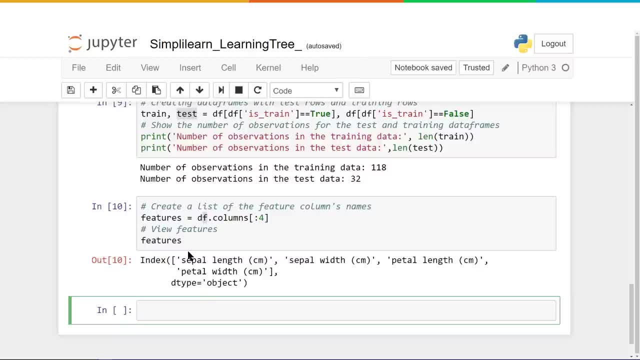 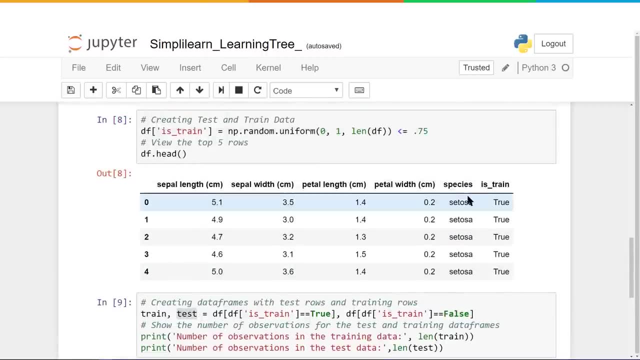 And so when I run this, you'll see down here that it creates an index: sepa length, sepa width, petal length and petal width. And this should be familiar because if you look up here, here's our column titles going across. 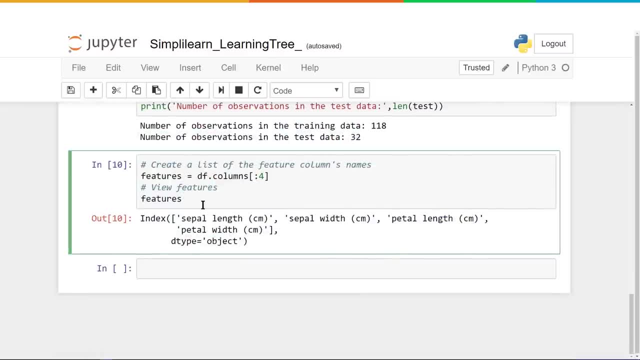 And here's the first four. One thing I want you to notice here is that when you're in a command line- whether it's Jupyter Notebook or you're running command line in the terminal window- if you just put the name of it it'll print it out. 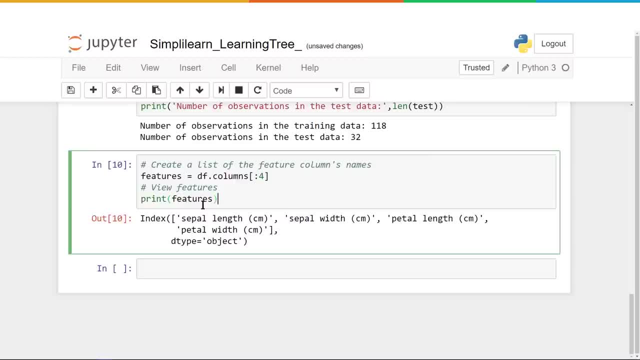 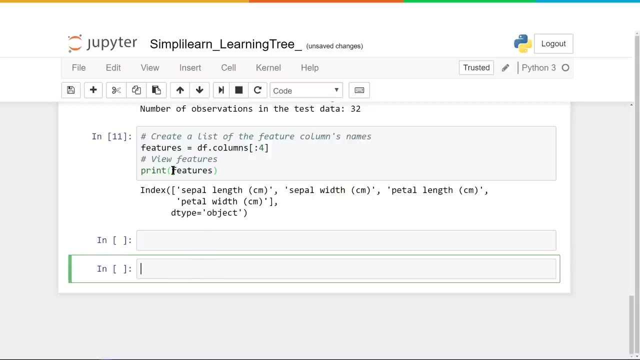 This is the same as doing print features And the shorthand is you just put features in here. If you're actually writing a code and saving the script and running it by remote, you really need to put the print in there. But for this, when I run it, you'll see it gives me the same thing. 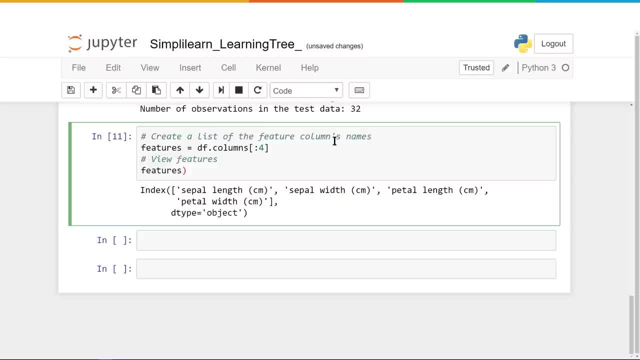 But for this we want to go ahead and we'll just leave it as features because it doesn't really matter. And this is one of the fun things about Jupyter Notebooks is I'm just building the code as we go, And then we need to go ahead and create the labels for the other part. So let's take a look and see what that looks like. So I'm going to go ahead and create the labels for the other part. For our final step, I'm going to go ahead and create the labels for the other part. For our final step, I'm going to go ahead and create the labels for the other part. 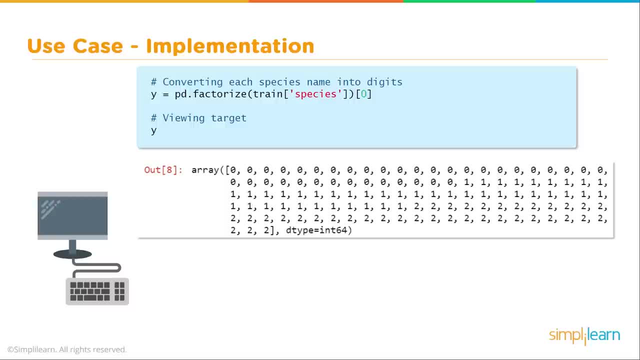 So our final step in prepping our data before we actually start running the training and the testing, is we're going to go ahead and convert the species on here into something the computer understands. So let's put this code into our script and see where that takes us. 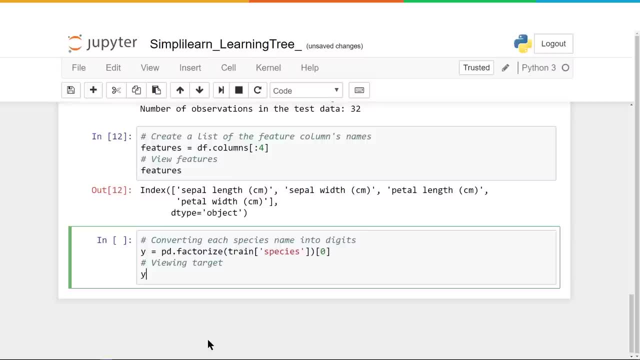 All right, here we go. We've set y equal to pdfactorize, train species of 0.. So let's break this down just a little bit. We have our pandas right here: pdfactorize What's factorize doing. I'm going to come back to that in just a second. 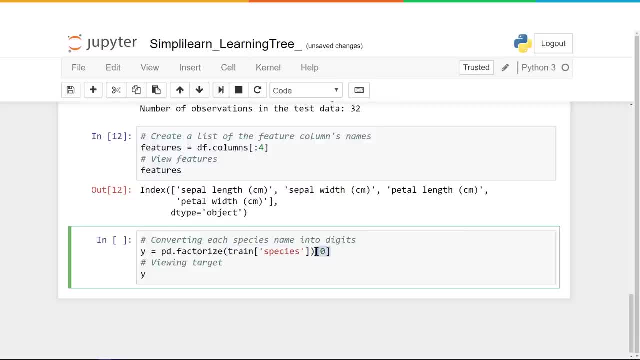 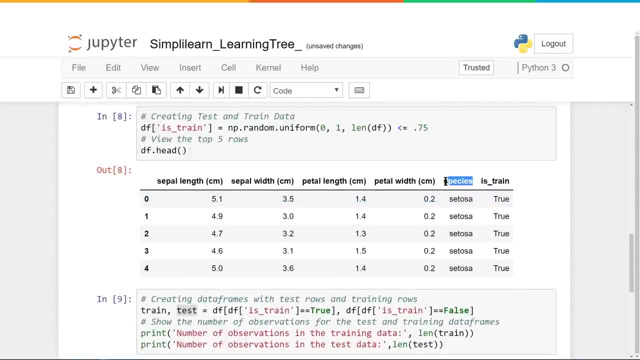 Let's look at what train species is and why. we're looking at the group 0 on there And let's go up here and here is our species. Remember this, that we created this whole column here for species And then it has setosa setosa, setosa, setosa. 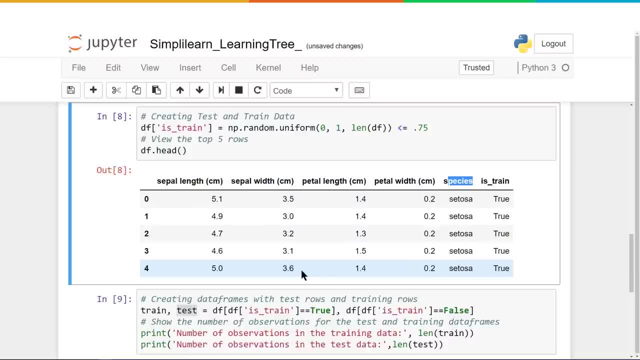 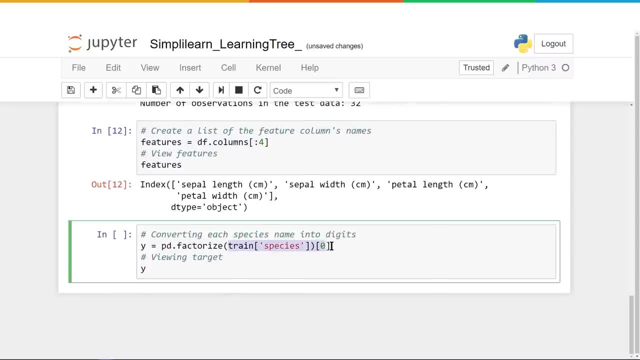 And if you scroll down enough, you'd also see virginica and vericolor. We need to convert that into something the computer understands: Zeros and ones, So the train species of 0, because this is in the format of an array of arrays. 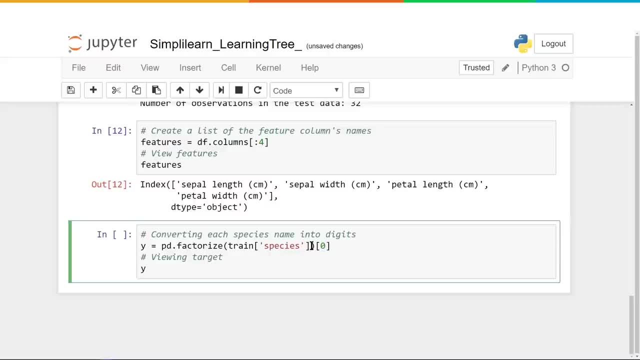 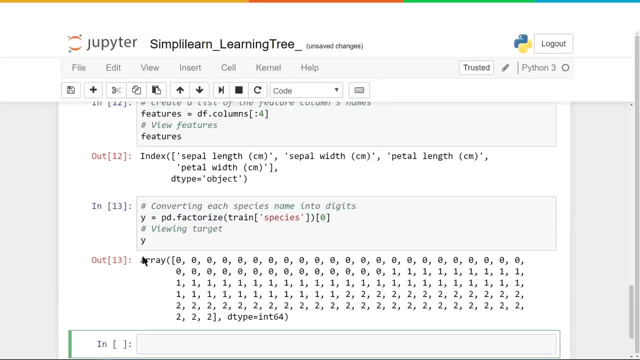 so you have to have the 0 on the end, And then species is just that column Factorize goes in there and looks at the fact that there's only three of them. So when I run this, you'll see that y generates an array that's equal to. 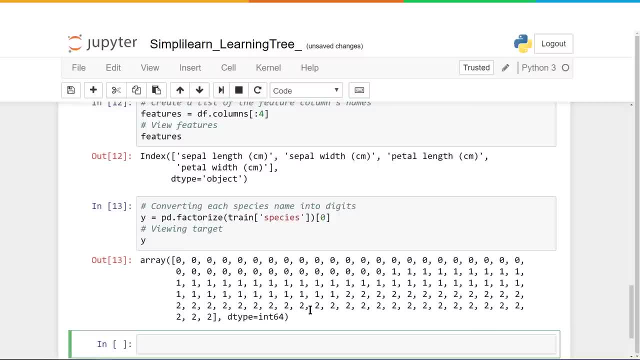 in this case it's a training set and it's zeros, ones and twos representing the three different kinds of flowers we have. So now we have something the computer understands and we have a nice table that we can read and understand. 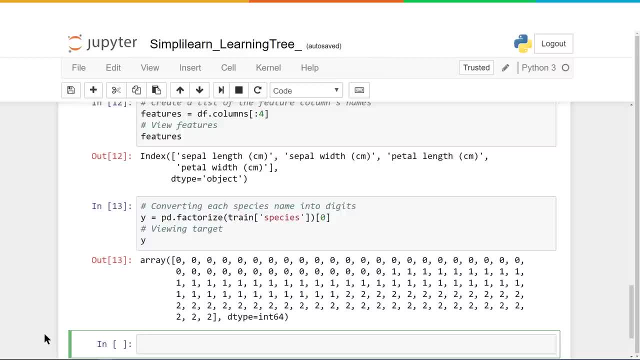 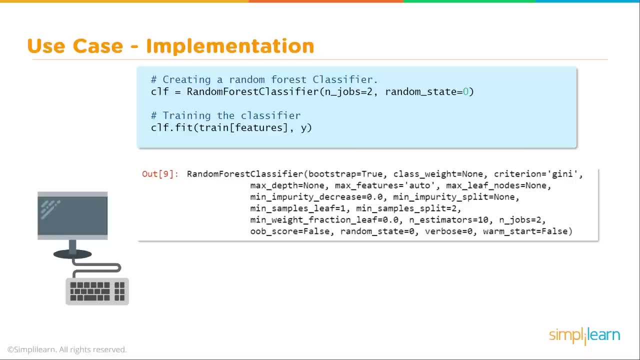 And now, finally, we get to actually start doing the predicting. So here we go. We have two lines of code. Oh, my goodness, that was a lot of work to get to two lines of code, But there is a lot in these two lines of code. 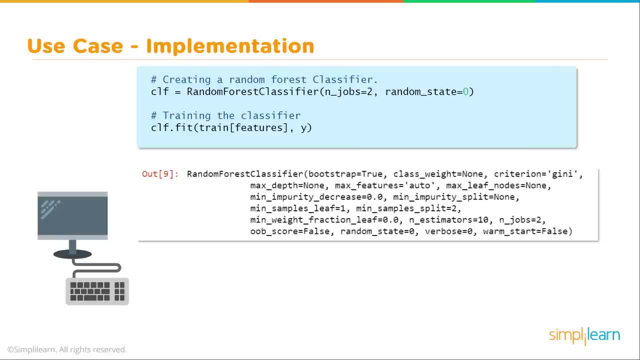 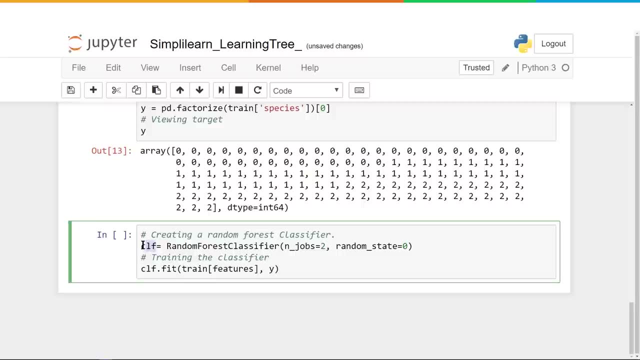 So let's take a look and see what's going on here. Put this into our full script that we're running And let's paste this in here And let's take a look and see what this is. We're creating a variable clf. 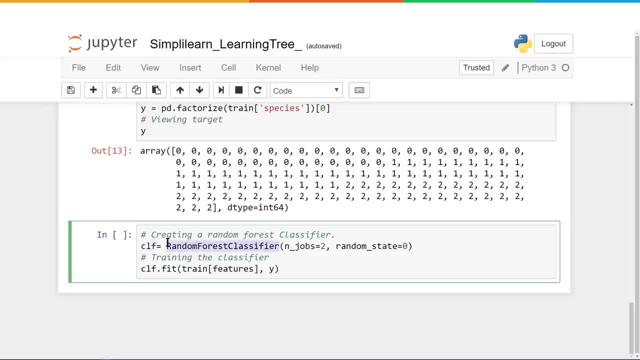 And we're going to set this equal to the random forest classifier And we're passing two variables in here And there's a lot of variables you can play with. As far as these two are concerned, they're very standard njobs. all that does is to prioritize it. 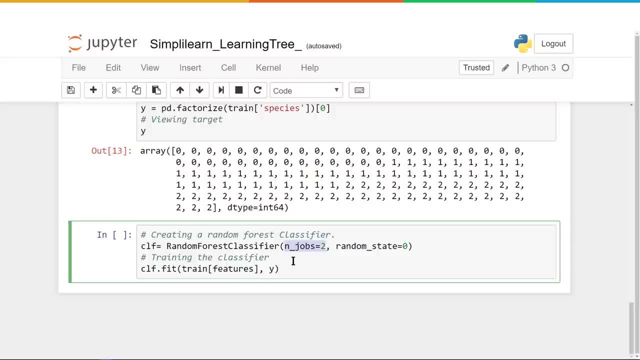 Not something to really worry about. Usually, when you're doing this on your own computer, you do njobs equals two If you're working in a larger or big data and you need to prioritize it differently. this is what that number does. It changes your priorities and how it's going to run across the system. 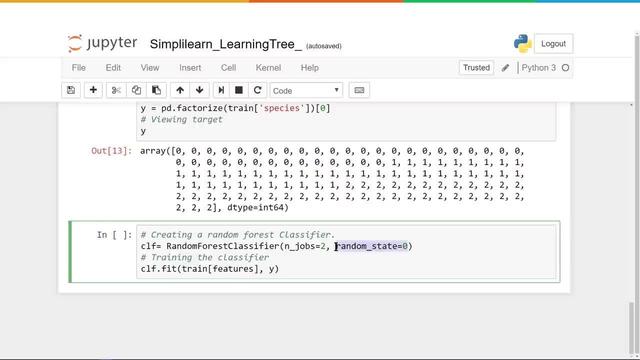 and things like that, And then the random state is just how it starts. Zero is fine for here, But let's go ahead and run this. We also have clffit train features y, And before we run it, let's talk about this a little bit more. 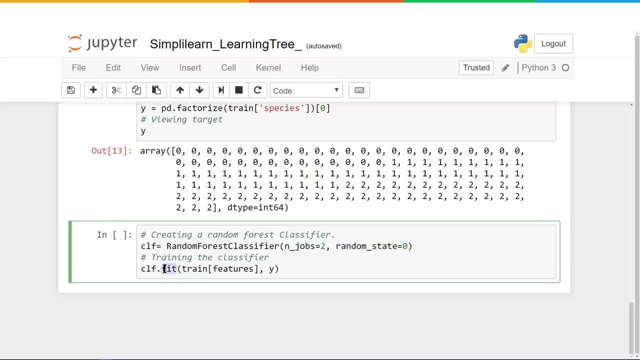 clffit. So we're fitting, we're training it. We are actually creating our random forest classifier right here. This is a code that does everything And we're going to take our training set. Remember, we kept our test off to the side. 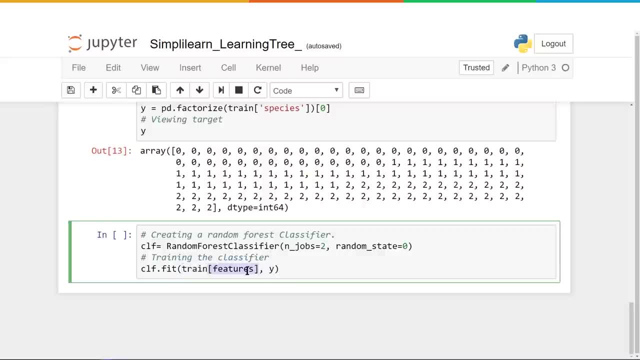 And we're going to take our training set with the features And then we're going to go ahead and put that in And here's our target, the y. So the y is zero, one and two that we just created And the features is the actual data going in. 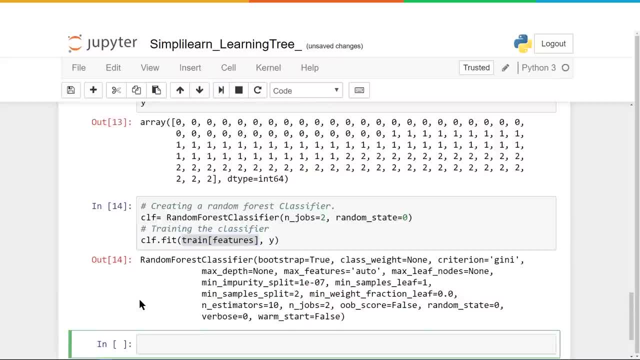 that we put into the training set And let's go ahead and run that. And this is kind of an interesting thing because it printed out the random forest classifier and everything around it. And so when you're running this in your terminal window or in a script like this, 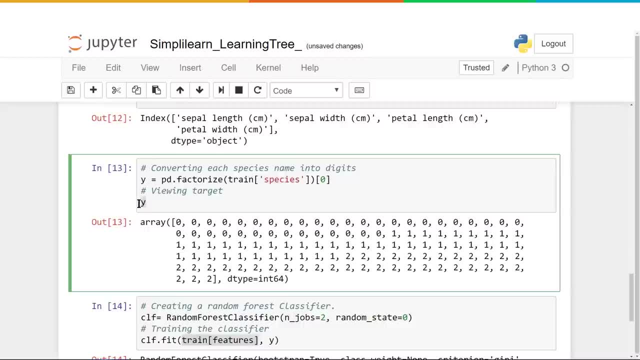 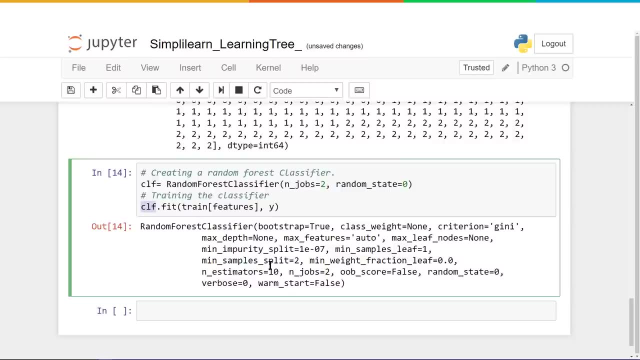 this automatically treats this, just like when we were up here and I typed in y and it printed out y instead of print y. This does the same thing: It treats this as a variable and prints it out. But if you were actually running your code, 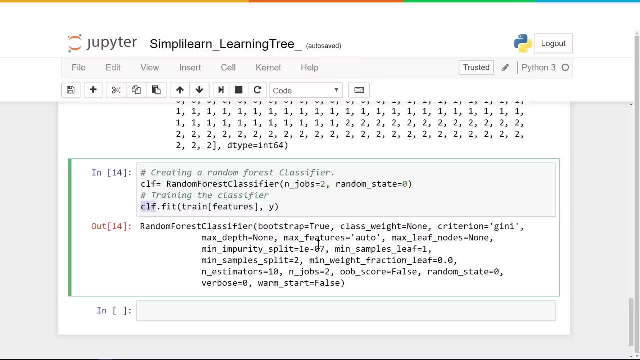 that wouldn't be the case And what it's printed out is. it shows us all the different variables we can change And if we go down here, you can actually see in jobs equals two. You can see the random state equals zero. Those are the two that we sent in there. 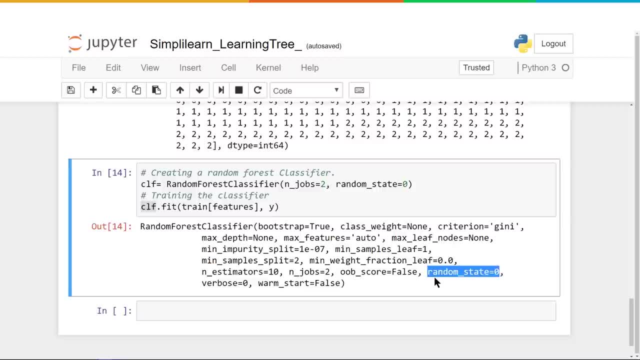 You would really have to dig deep to find out all these different meanings of all these different settings on here. Some of them are self-explanatory if you kind of think about it a little bit. like max features is auto, So all the features that we're putting in there. 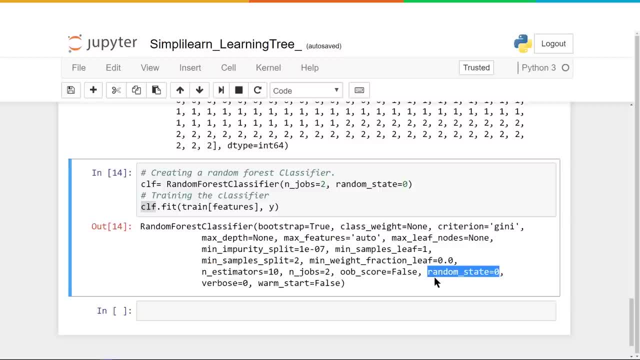 is just going to automatically take all four of them. Whatever we send it, it'll take. Some of them might have so many features because you're processing words. there might be like 1.4 million features in there, like multiple documents. 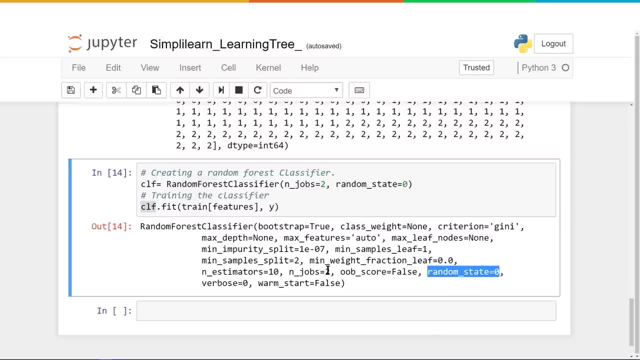 and that's how many different words are in there. At that point you probably want to limit the maximum features that you're going to process And leaf nodes- that's the end nodes. Remember we had the fruit and we're talking about the leaf nodes. 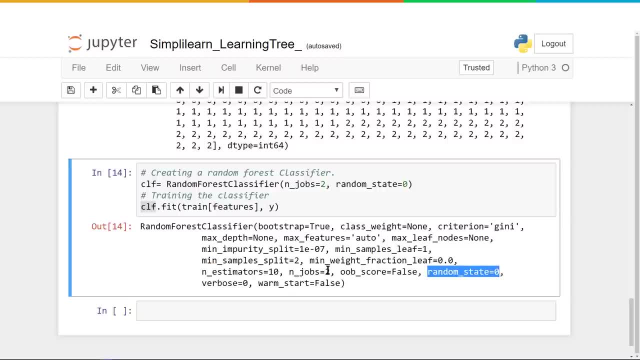 Like I said, there's a lot in this. We're looking at a lot of stuff here, So you might have- in this case there's probably only, I think- three leaf nodes, maybe four. You might have thousands of leaf nodes. 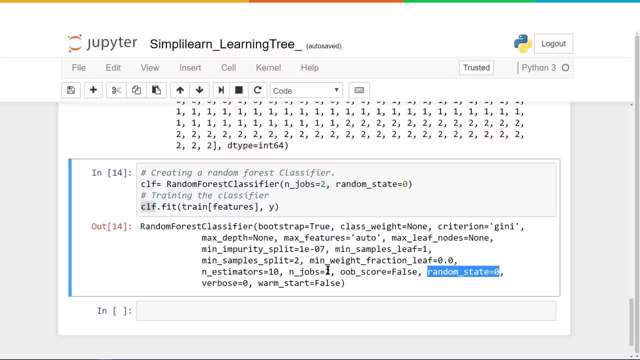 at which point you do need to put a cap on that and say, okay, you can only go so far, but you can only go so far. So what we're going to do now is limiting the process and making sure we don't overwhelm a system. 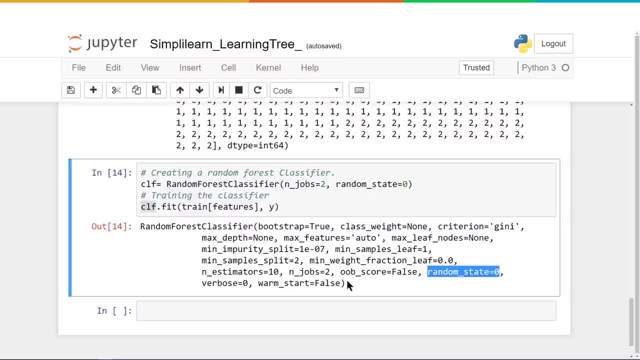 And there's some other settings in here. Again, we're not going to go over all of them. Warm start equals false, Warm start is if you're programming it one piece at a time externally. Since we're not, we're not going to have. 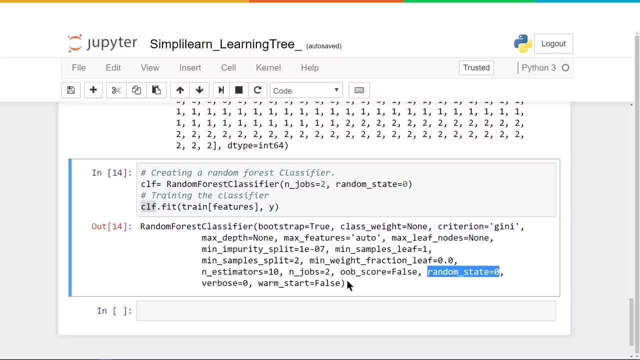 we're not going to continually detrain this particular learning tree And again, like I said, there's a lot of things in here that you'll want to look up in more detail from the sklearn, but what we want to do is fit or train our features. 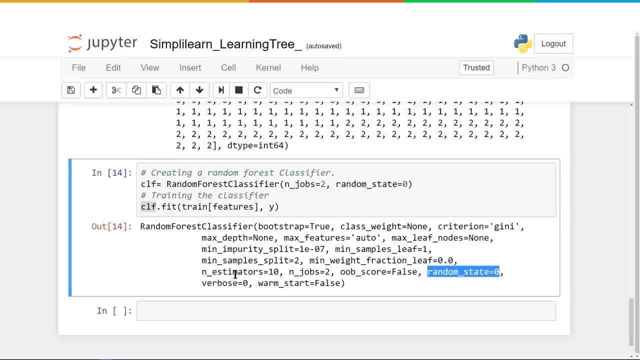 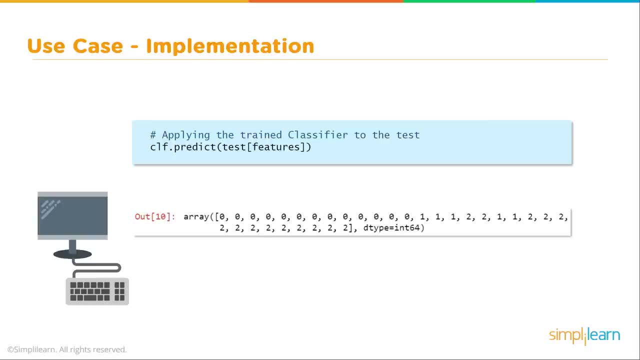 and our target Y. So now we have our training model. what's next? If we're going to create a model, we now need to test it. Remember we set aside the test feature, test group- 25% of the data. 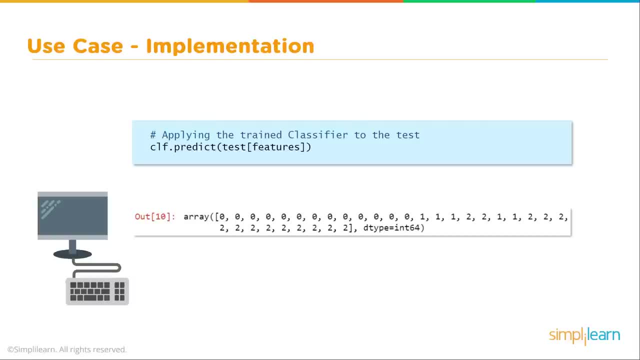 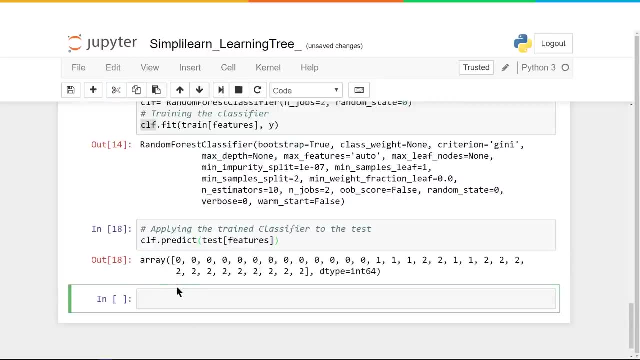 So let's go ahead and take this code and let's put it into our script and see what that looks like. Okay, here we go And we're going to run this And it's going to come out with a bunch of zeros, ones and twos. 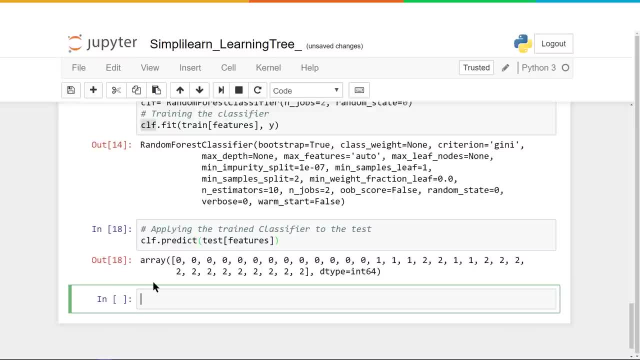 Which represents the three types of flowers: The setosa, the virginica and the versicolor. And what we're putting into our predict is the test features, And I always kind of like to know what it is I am looking at. So real quick. 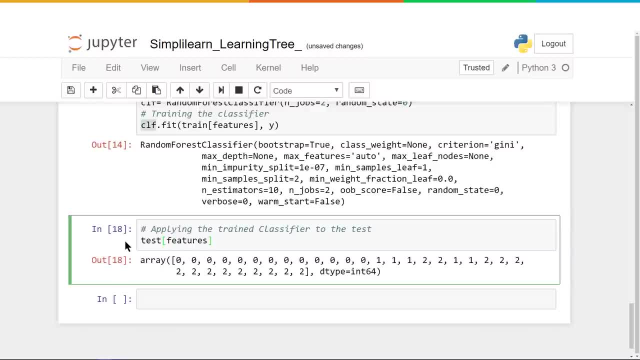 we're going to do test features And remember. features is an array of sepal length, sepal width, petal length, petal width. So when we put it in this way, it actually loads all these different columns that we're going to be using. 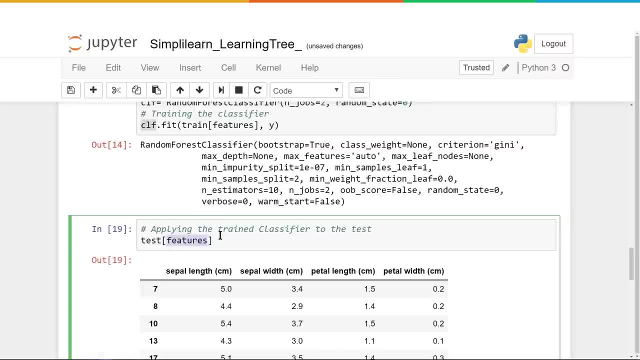 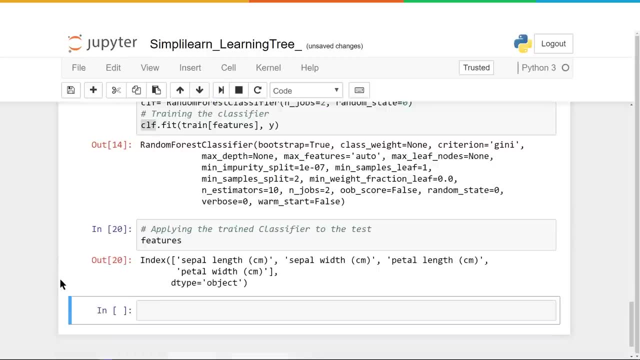 for our model. These are the columns that we loaded into features. So if we did just features, let me just do features in here and see what features looks like. This is just playing with Panda's data frames. You'll see that it's an index. 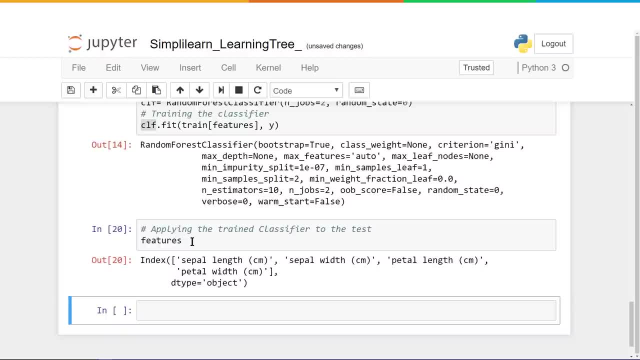 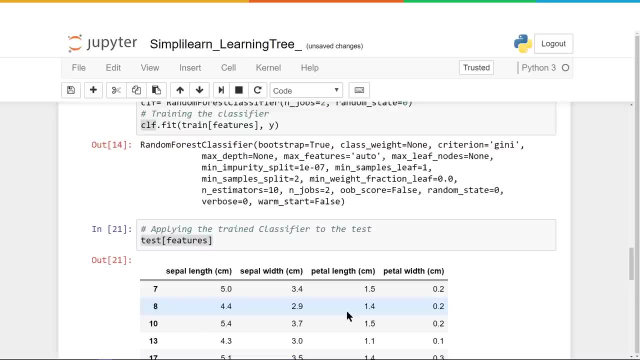 So when you put an index in like this into test features, into test, it then takes those columns and creates a Panda data frame from those columns And in this case we're going to go ahead and put those in. So we're going to put each one of these lines. 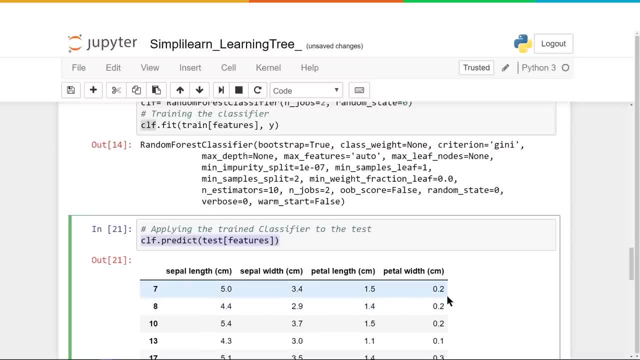 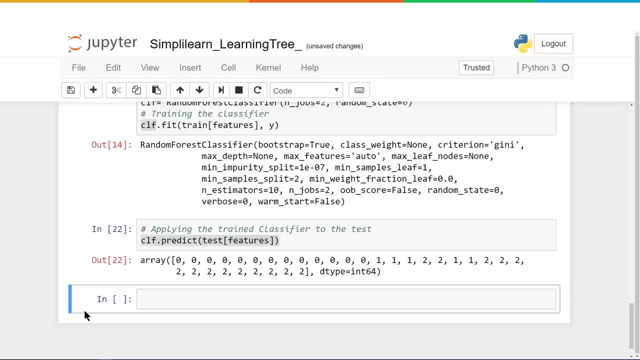 of data- the 5.0,, 3.4,, 1.5,, .2, and we're going to put those in and we're going to predict what our new forest classifier is going to come up with. And this is what it predicts. It predicts: 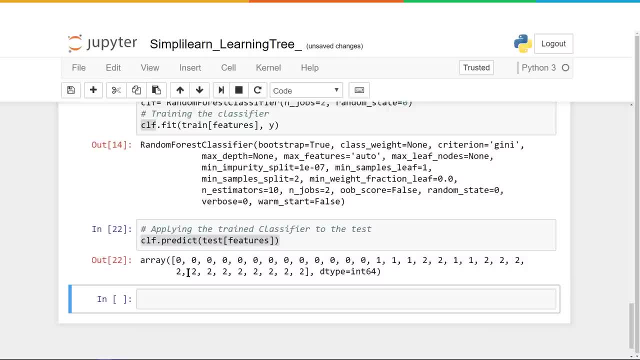 0,, 0,, 0,, 1,, 2,, 1,, 1,, 2,, 2,, 2, and again, this is the flower type: setosa virginica and versicolor. So now, 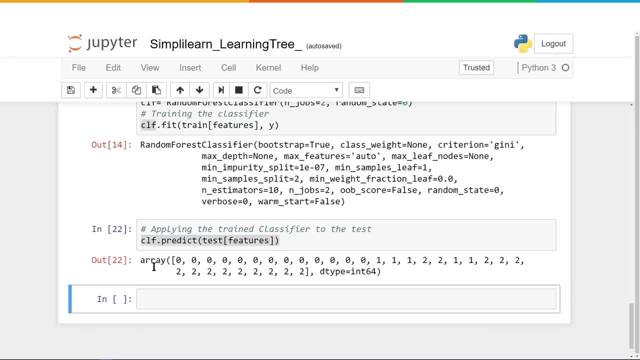 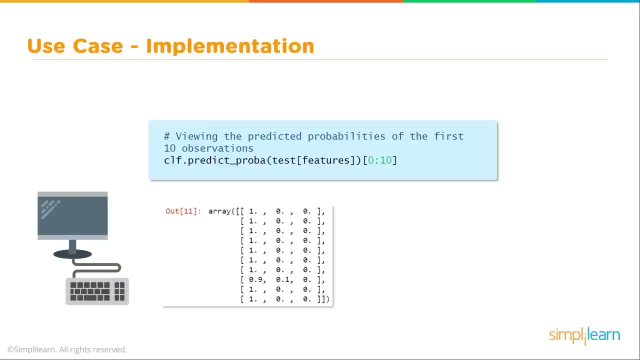 that we've taken our test features. let's explore that. Let's see exactly what that data means to us. So the first thing we can do with our predicts is we can actually generate a different prediction model. When I say different, we're going to view it differently. 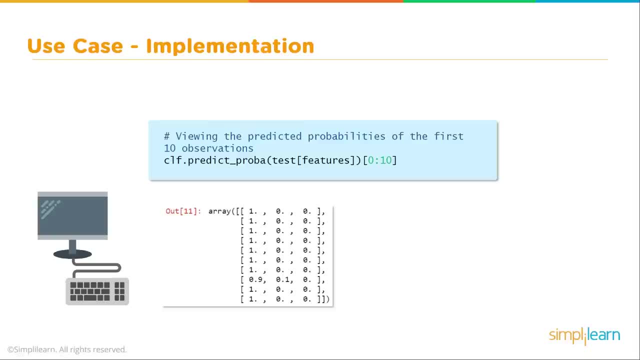 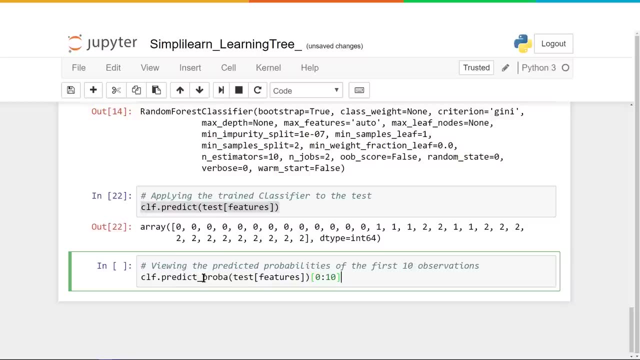 It's not that the data itself is different. So let's take this next piece of code and put it into our script. So we're pasting it in here and you'll see that we're doing predict and we've added underscore proba for probability. 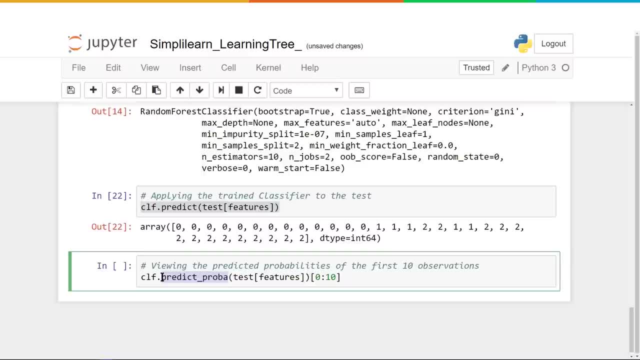 So there's our clfpredict probability. So we're running it just like we ran it up here, but this time, with this, we're going to get a slightly different result And we're only going to look at the first 10.. 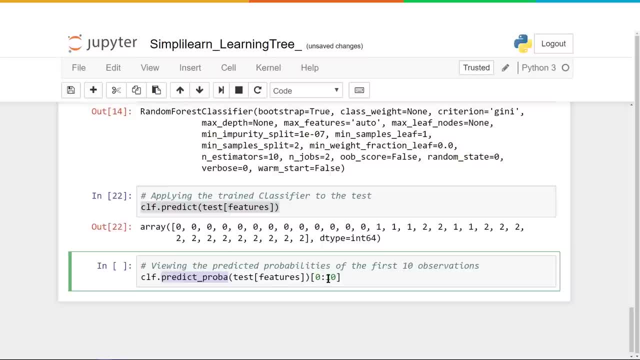 So you'll see down here, instead of looking at all of them, which was 27,- you'll see right down here that this generates a much larger field on the probability And let's take a look and see what that looks like and what that means. 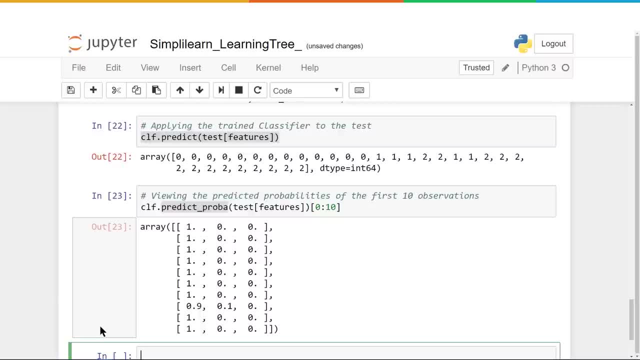 So when we do the predict underscore proba for probability, it generates three numbers. So we had three leaf nodes at the end And if you remember from all the theory we did, this is the predictors. The first one is predicting a 1 for setosa. 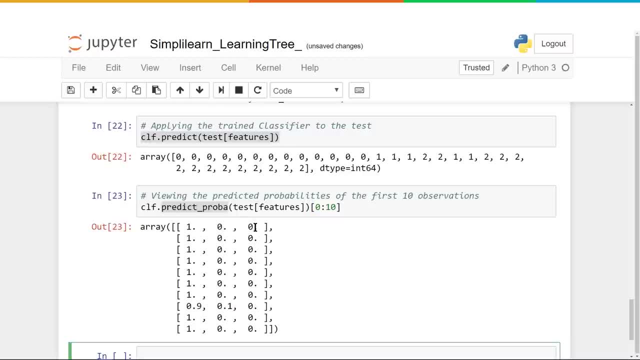 it predicts a 0 for virginica, and it predicts a 0 for versicolor, and so on, and so on, and so on. And let's you know what, I'm going to change this just a little bit. Let's look at 10. 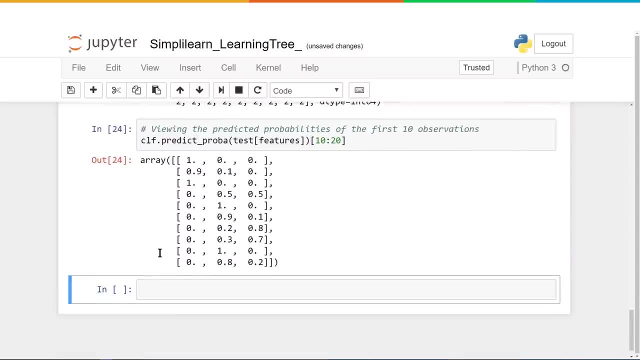 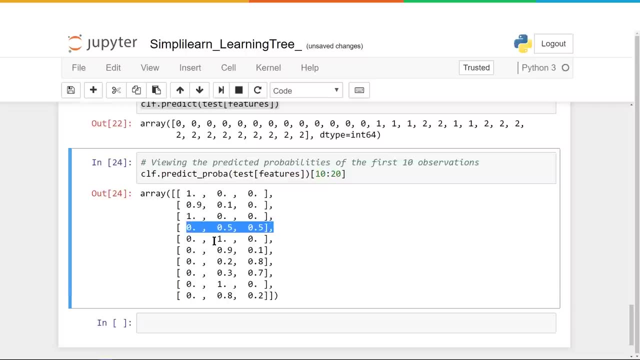 to 20, just because we can, And we start to get a little different of data and you'll see right down here it gets to this one, this line right here, And this line has 0, 0.5,, 0.5.. 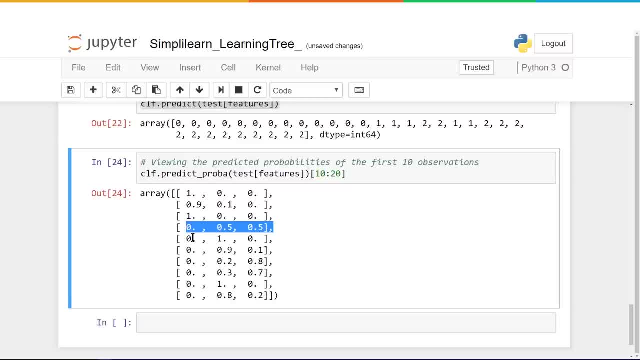 And so if we're going to vote and we have two equal votes, it's going to go with the first one. So it says: setosa gets 0 votes, virginica gets 0.5 votes, versicolor gets 0.5. 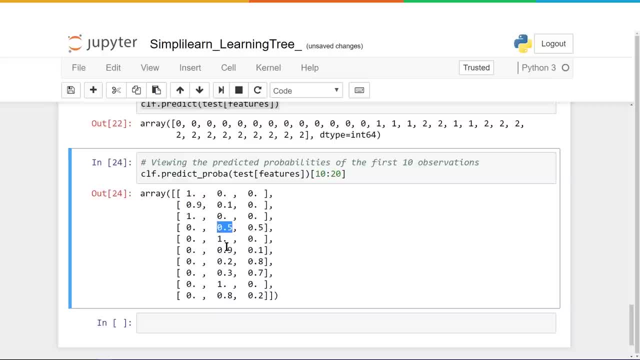 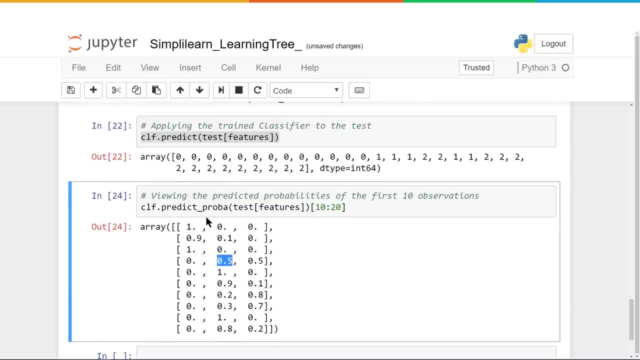 votes, but let's just go with the virginica, since these two are equal, And so on and so on. down the list You can see how they vary on here. So now we've looked at both how to do a basic predict of the features- and we've 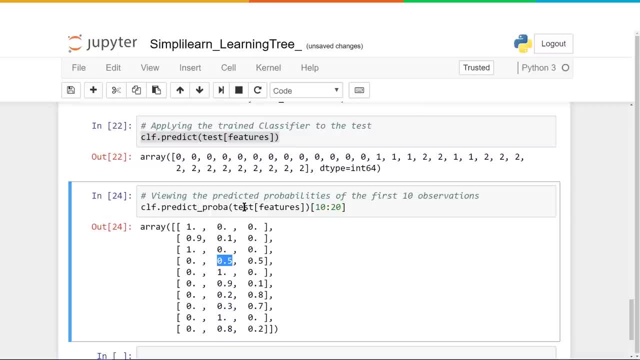 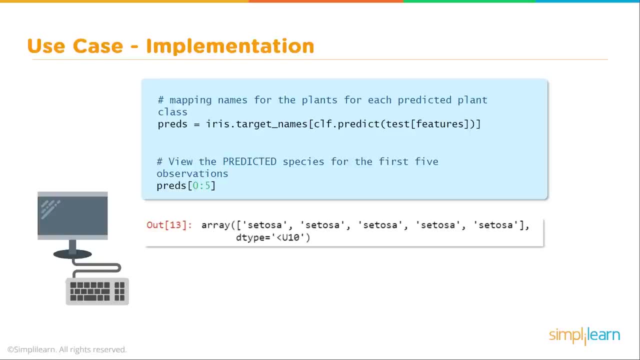 looked at the predict probability. Let's see what's next on here. So now we want to go ahead and start mapping names for the plants. We want to attach names so that it makes a little more sense for us, And that's what we're going to do in these next two steps. 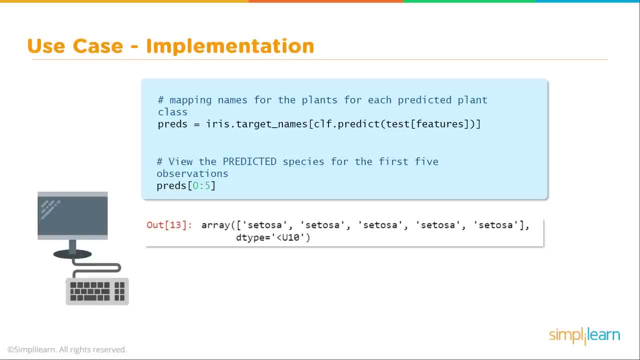 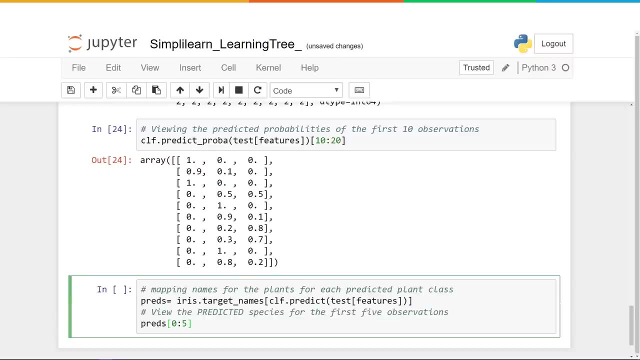 We're going to start by setting up our predictions and mapping them to the names. So let's see what that looks like And let's go ahead and paste that code in here and run it. And this goes along with the next piece of code. 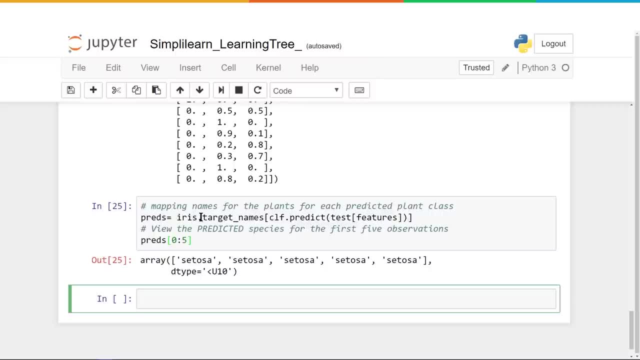 So we'll skip through this quickly and then come back to it a little bit. So here's iristargetNames And, if you remember correctly, this was the names that we've been talking about this whole time: The setosa virginica versicolor. 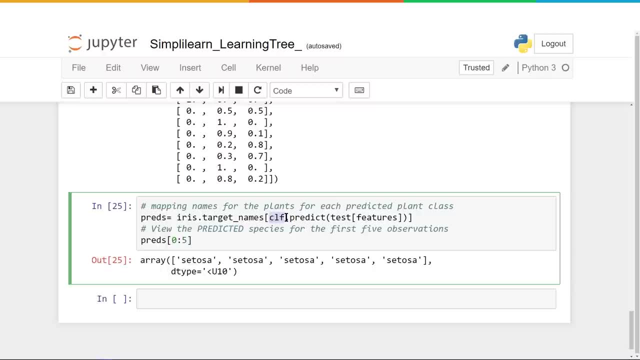 And then we're going to go ahead and do the prediction again. We could have just set a variable equal to this instead of re-running it each time, But we're going to run it again. clfpredictTestFeatures: Remember that returns the zeros. 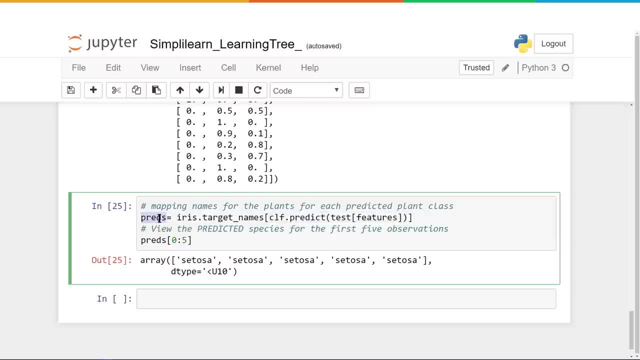 the ones and the twos, And then we're going to set that equal to prediction and predictions. So this time we're actually putting it in a variable And when I run this, it distributes and it comes out as an array And the array is setosa, setosa. 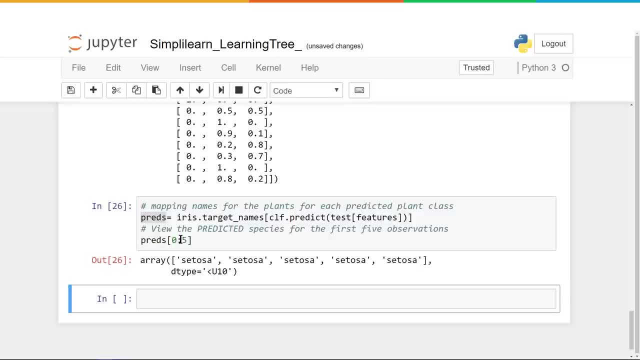 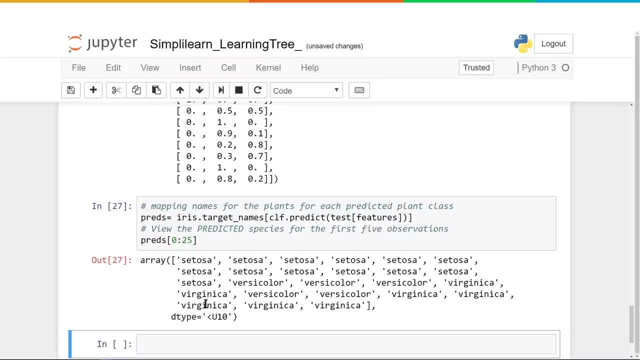 setosa, setosa, setosa. We're only looking at the first five. We could actually do. let's do the first 25 just so we can see a little bit more on there, And you'll see that it starts mapping it to all the different flower types. 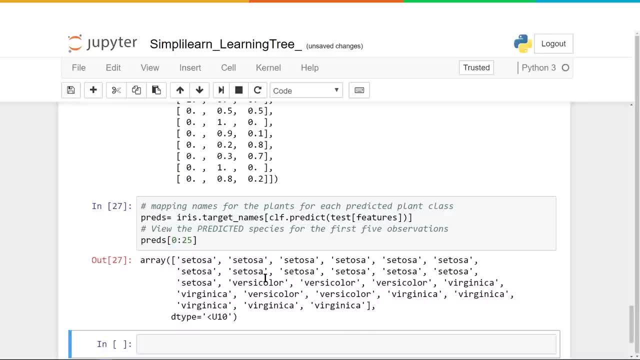 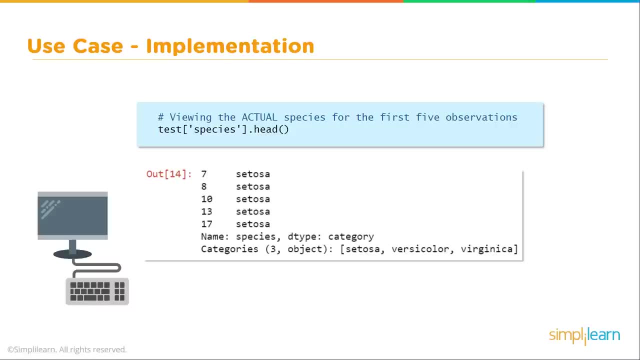 The versicolor and the virginica in there And let's see how this goes with the next one. So let's take a look at the top part of our species in here And we'll take this code and put it in our script. 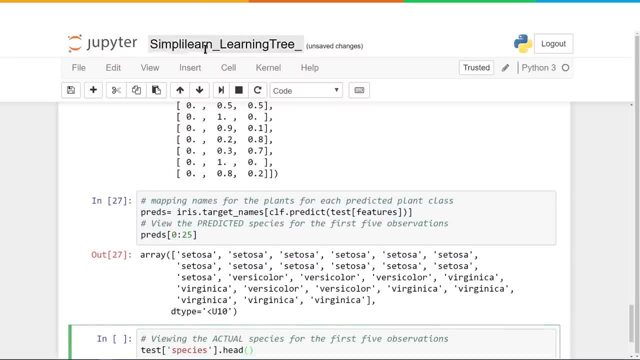 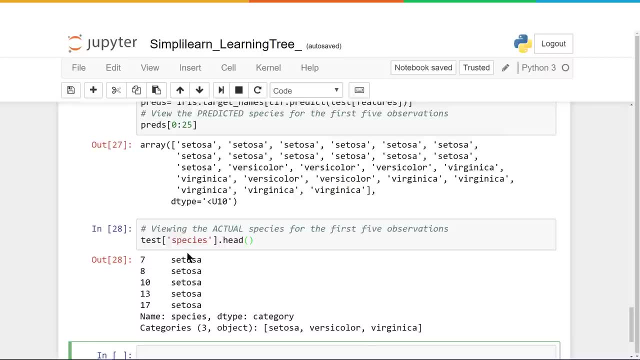 And let's put that down here and paste it. There we go And we'll go ahead and run it. And let's talk about both these sections of code here And how they go together. The first one is our predictions, And I went ahead. 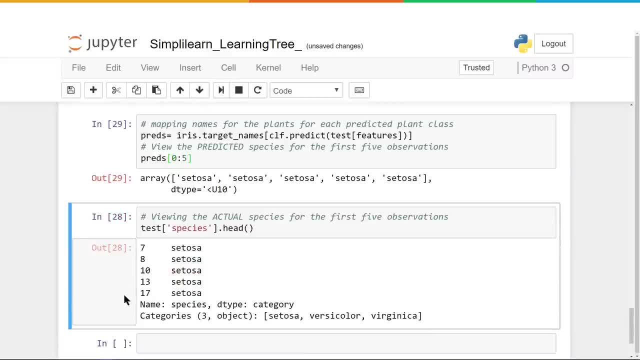 and did predictions through 25.. Let's just do 5. And so we have setosa, setosa, setosa, setosa. That's what we're predicting from our test model. And then we come down here and we look at test species. 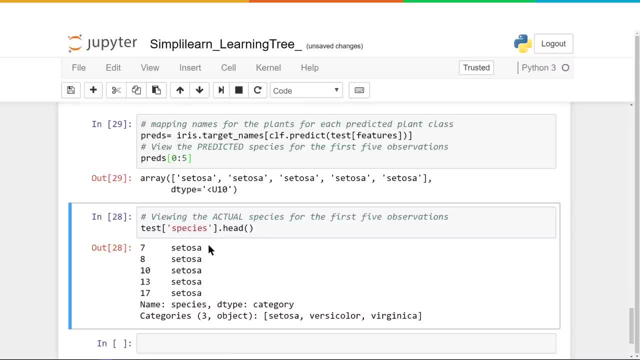 I remember I could have just done testspecieshead And you'll see it says setosa, setosa, setosa, setosa And they match. So the first one is what our forest is doing And the second one is what the actual data is Now. 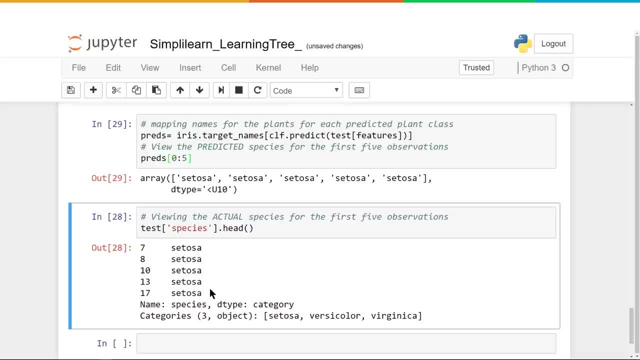 we need to combine these so that we can understand what that means. We need to know how good our forest is, How good it is at predicting the features. So that's where we come up to the next step, Which is lots of fun. 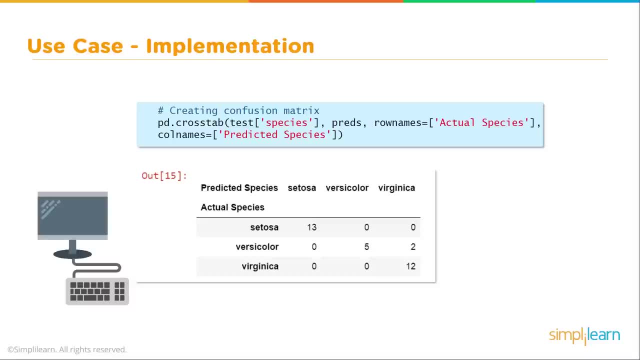 We're going to use a single line of code to combine our predictions and our actuals. So we have a nice chart to look at And let's go ahead and put that in our script in our Jupyter notebook. here Let's see. 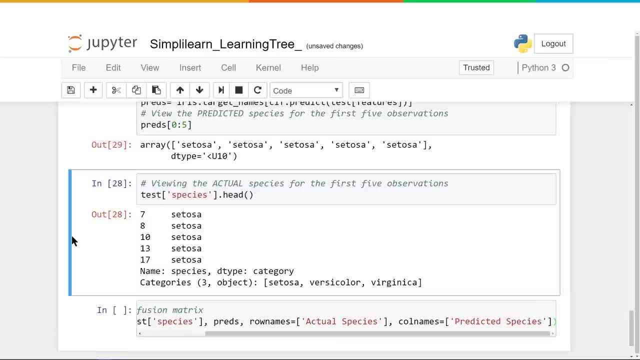 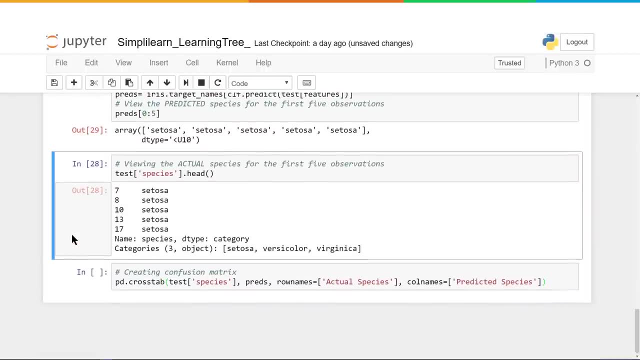 Let's go ahead and paste that in, And then I'm going to, because I'm on the Jupyter notebook- I can do a control minus. You can see the whole line there. There we go, Resize it And let's take a look and see. 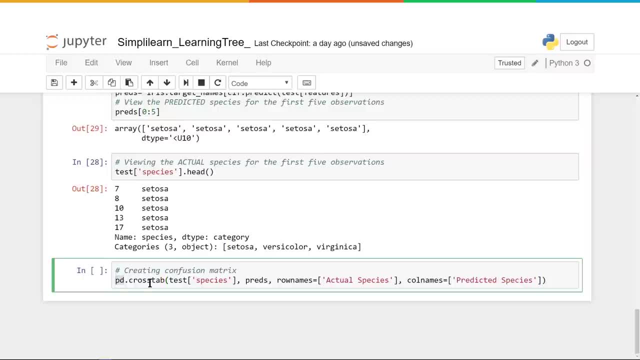 what's going on here. We're going to create in pandas- Remember, pd stands for pandas And we're doing a crosstab. This function takes two seconds to create two sets of data and creates a chart out of them. So when I run it you'll get a nice chart down here. 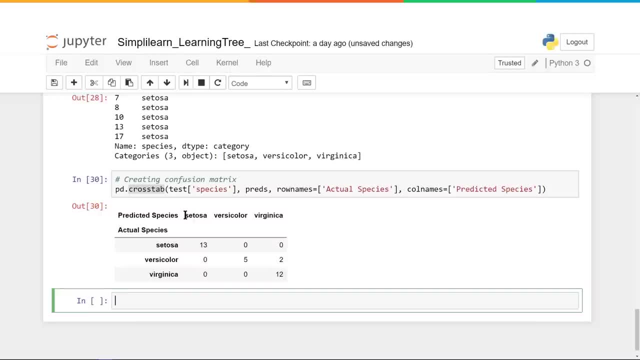 And we have the predicted species. So across the top you'll see the setosa versicolor virginica And the actual species, Setosa versicolor virginica. And so the way to read this chart and let's go ahead and take a look. 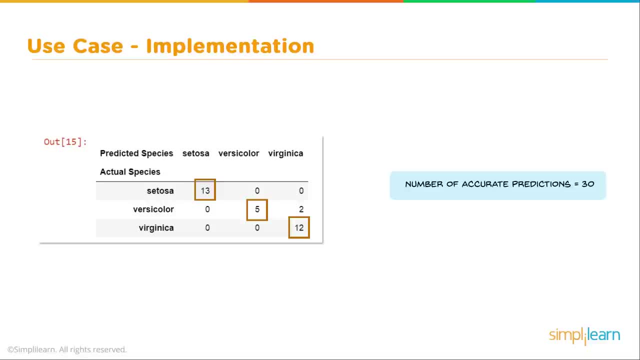 on how to read this chart here. When you read this chart, you have setosa where they meet, You have versicolor where they meet And you have virginica where they meet, And they're meeting where the actual and the predicted agree. 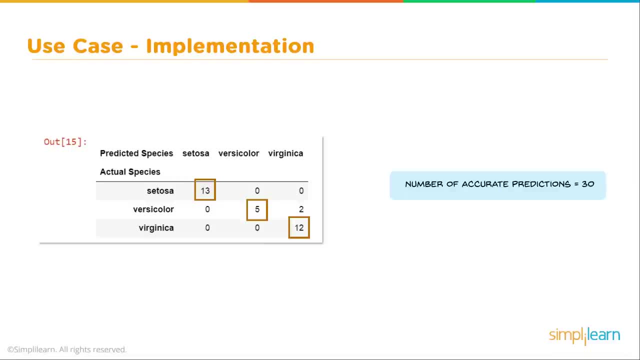 So this is the number of accurate predictions. So in this case it equals 30. If you add 13 plus 5 plus 12, you get 30. And then we notice here where it says virginica, but it was supposed to be versicolor. 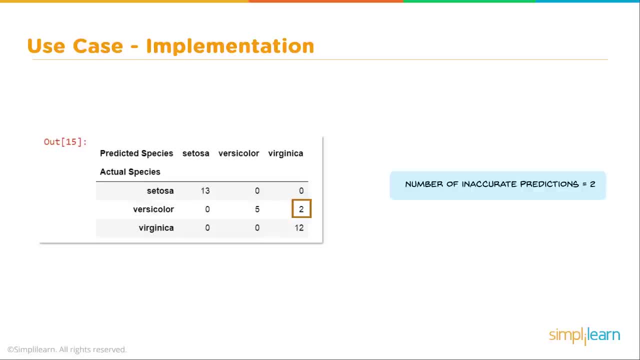 This is inaccurate. So now we have two: Two inaccurate predictions and 30 accurate predictions. So we'll say that the model accuracy is 93. That's just 30 divided by 32. And if we multiply it by 100, we can say that it is. 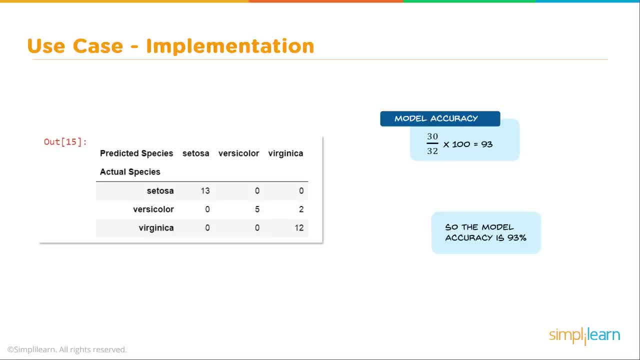 93% accurate. So we have a 93% accuracy with our model. I did want to add one more quick thing in here on our scripting before we wrap it up, So let's flip back on over to my script In here. we're going to take this: 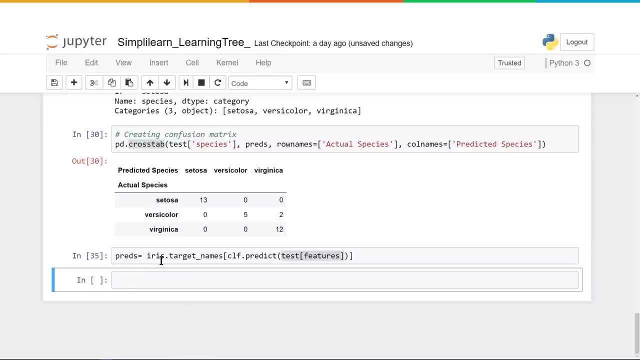 line of code from up above. I don't know if you remember it, but predicts equals the iris dot target underscore names. So we're going to map it to the names And we're going to run the prediction And we read it on test features. But 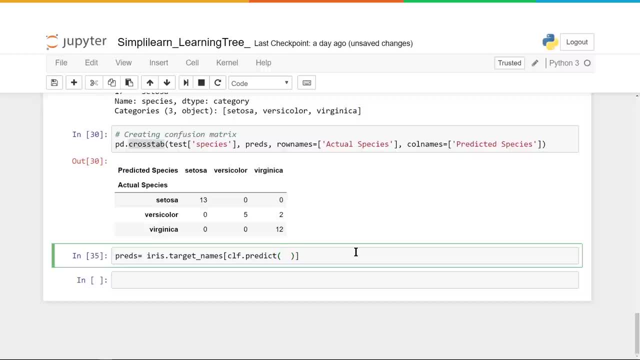 you know, we're not just testing it, We want to actually deploy it. So at this point I would go ahead and change this, And this is an array of arrays. This is really important when you're running these to know that. So you need the double. 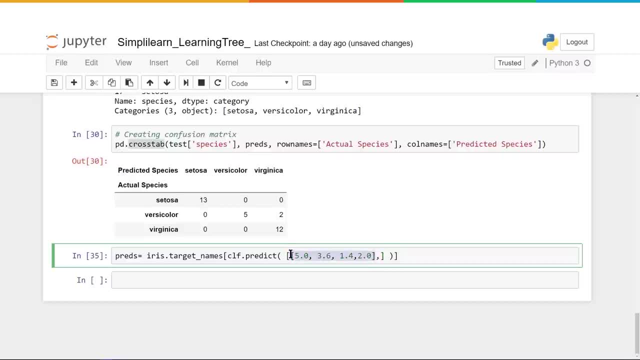 brackets And I could actually create data. maybe let's just do two flowers, So maybe I'm processing more data coming in And we'll put two flowers in here, And then I actually want to see what the answer is. So let's go ahead and. 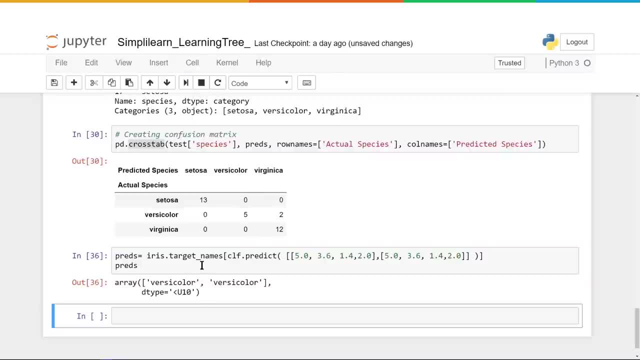 type in preds and print that out, And when I run this you'll see that I've now predicted two flowers that maybe I measured in my front yard as versicolor and versicolor- Not surprising, since I put the same data in for each one. This would be the. 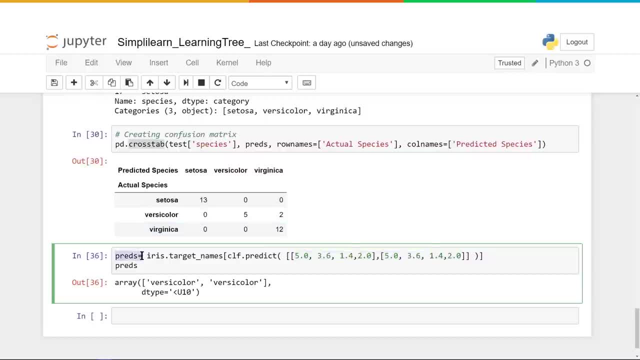 actual end product going out to be used on data that you don't know the answer for. So that's going to conclude our scripting part of this, And let's just go ahead and take a look at the key takeaways. with today's tutorial, We have solutions.